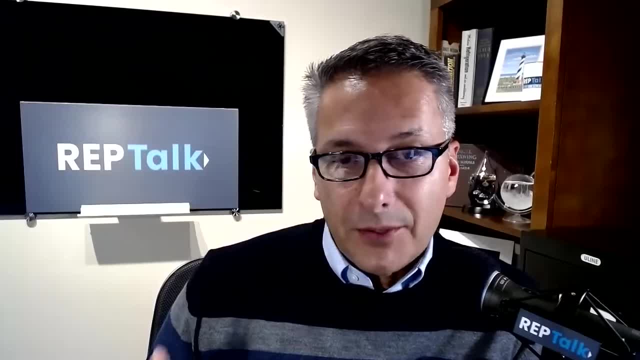 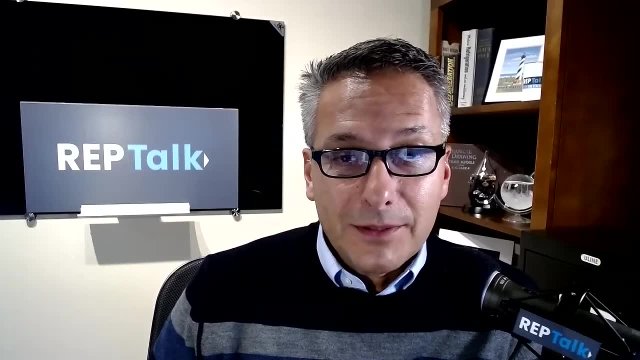 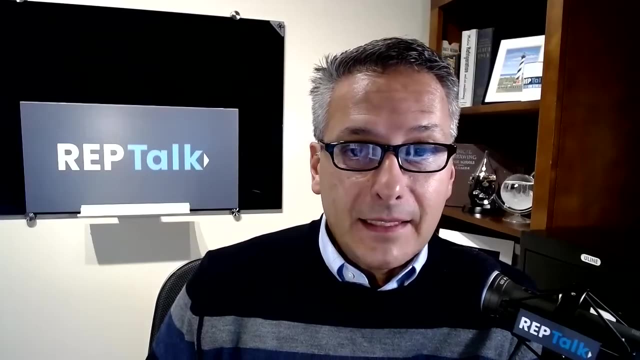 So always a concern. Next, there's odors, and odors fall under gases as well. These could be volatile organic compounds. new carpet smell, new car smell- Those are examples of violent VOCs. In fact, formaldehydes coming out of new construction materials are often a problem as well. 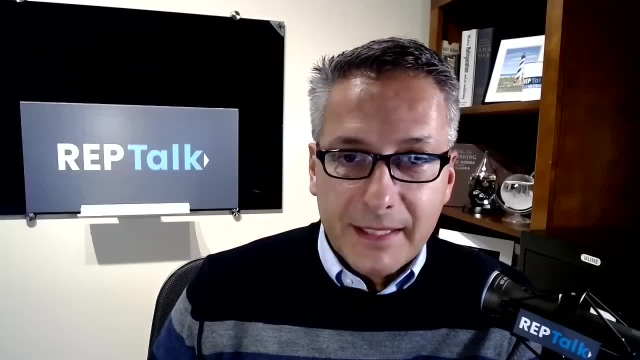 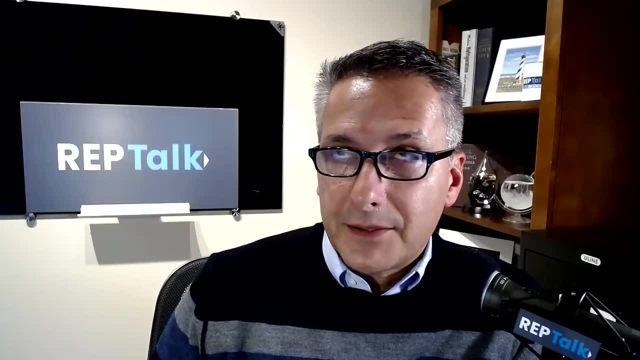 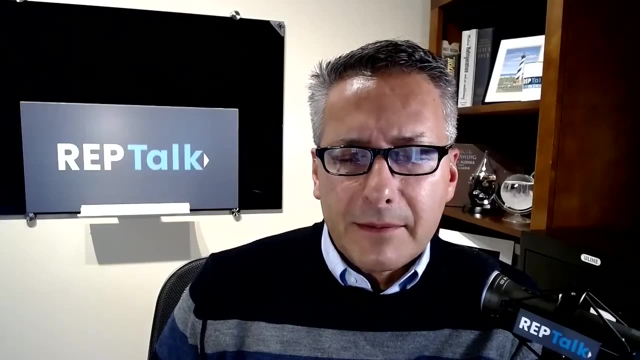 And pet odors And finally, particulates. Particulates can be- these are all the things suspended in the air. They're so light in weight they're suspended in the air for various times, depending on the actual particulate we're talking about. But anyway, these would be things. 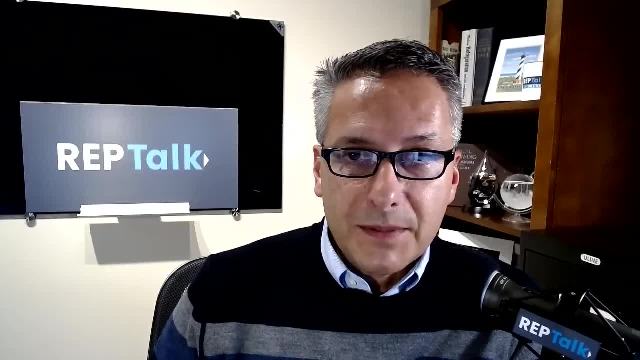 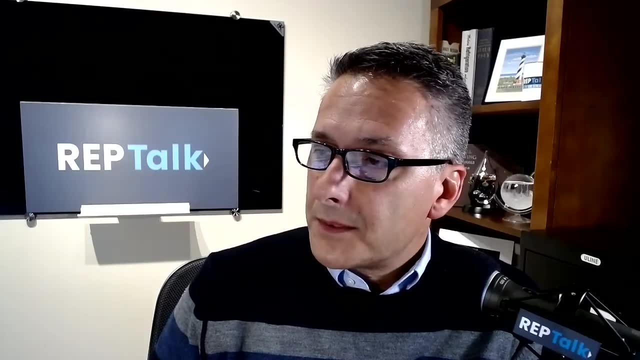 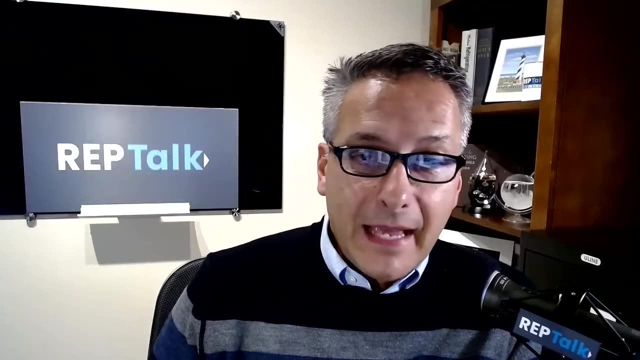 we can't see over 99% of them, by the way, either, So most of them are invisible to our naked eyes. Things like dust particles, smoke particles, pollen. So this is where the allergy sufferers of the world live- Animal dander, Actually, and human dander as well. Dander, by the way, is just a fancy word for dead. 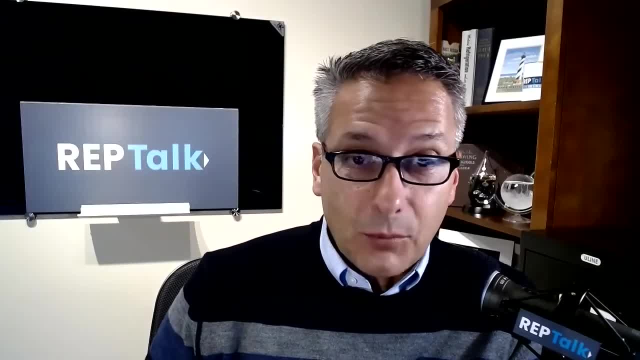 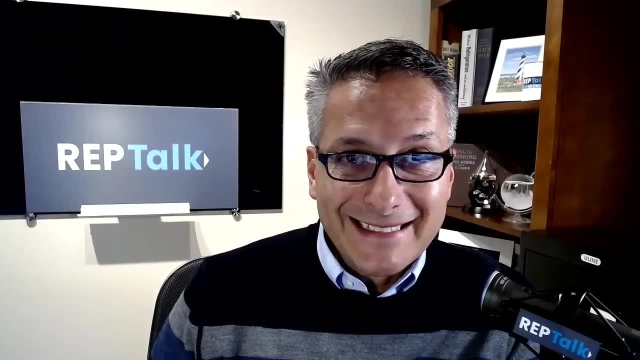 skin cells. You know, I think of the word dandruff, right? So not only animals, but humans. we are some of the worst offenders when it comes to shedding dead skin cells, And you know, when we shed, or when pets shed, they have to go somewhere, right? 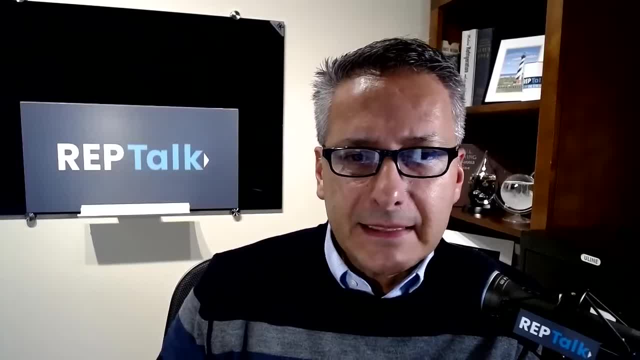 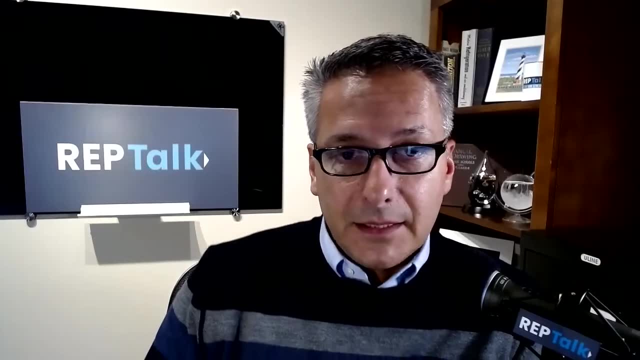 And dust mites, Dust mites. the big issue with dust mites is what they leave behind And, as disgusting as it might sound, it's dust mite fecal matter And it's very allergenic. So think about it the next time you empty out the vacuum canister. You know you're actually in. 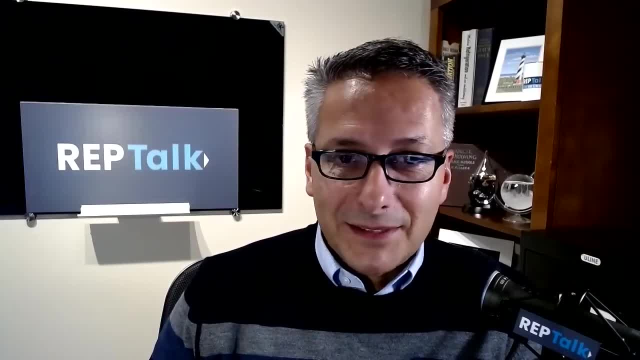 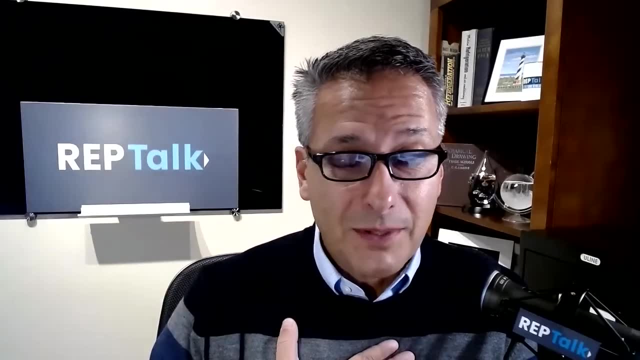 there, right, Part of you is in there. I know it sounds gross, but that's just the fact of life, right? So these are the things that are in and we live in and around and we actually cause to create. So we're actually sources of pollution ourselves, really just by breathing. I forget what. 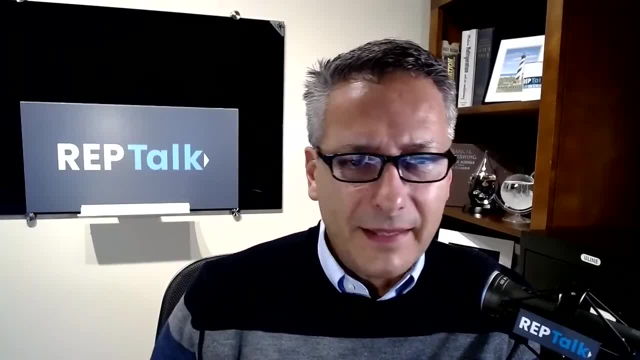 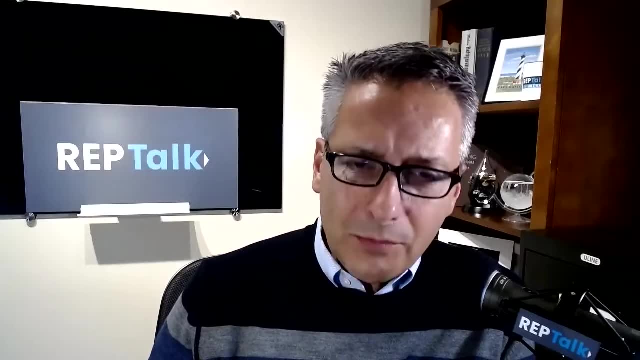 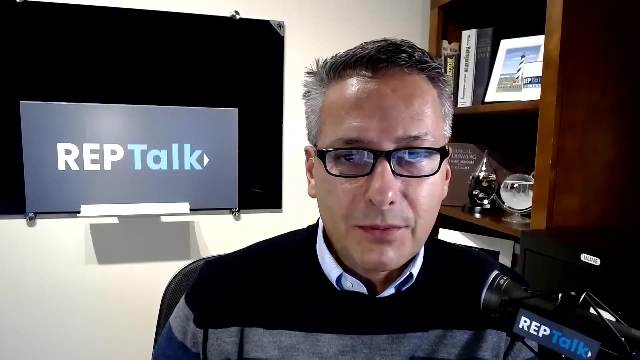 actual number is. but every breath, every exhale that we have, we give off. I think it's like something over 200 VOCs ourselves just by living and breathing. So those three categories of pollutants is what we're after: to try to reduce or I can't really say eliminate. 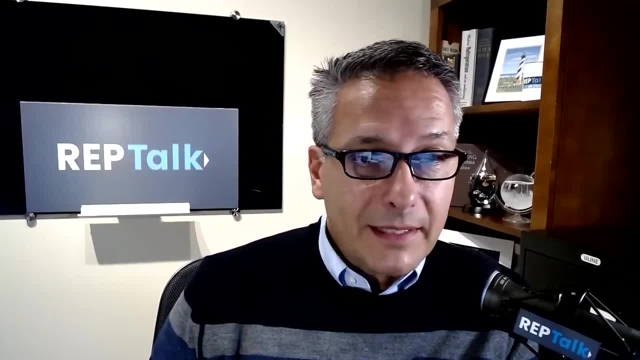 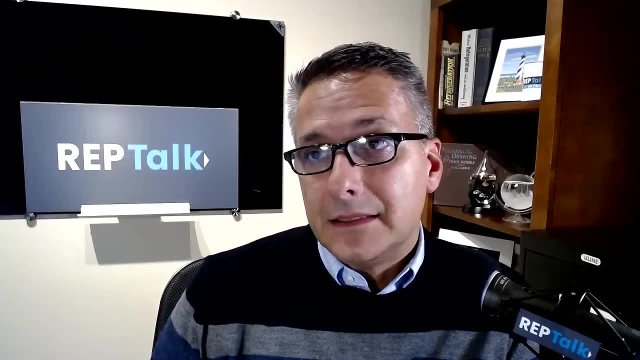 but reduce so we actually can breathe healthier, better, cleaner air in our spaces, our living spaces. right, We spend over 90% of our times indoors and, you know, the one space that we really have control over, when we want to take control over the breathing air, is our home. It's probably 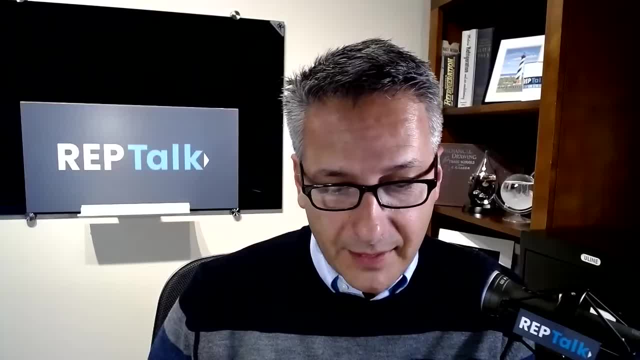 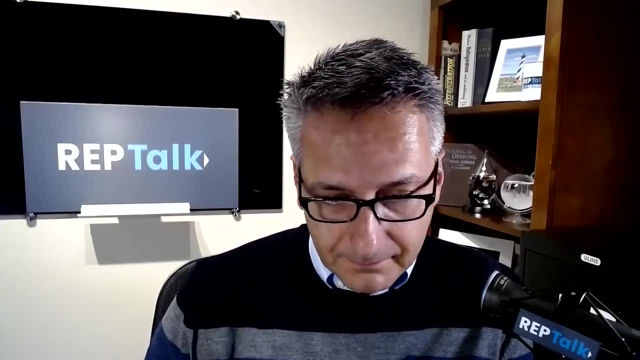 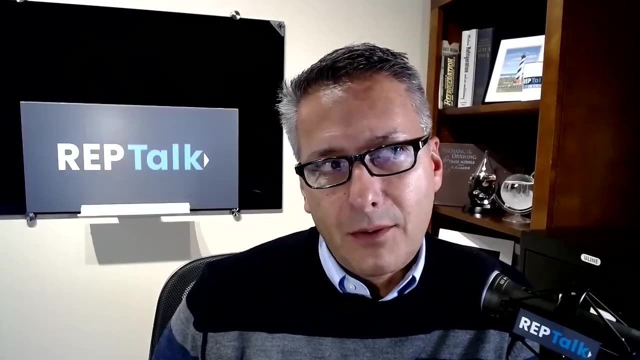 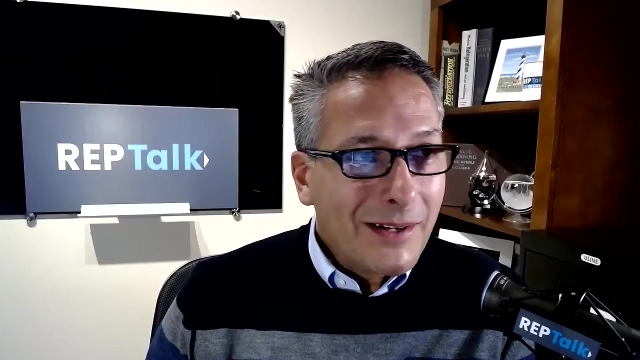 the only place we have control over our breathing air is in the house. So today I'd like to talk to you about some of those clean air strategies. So what I mean by that is the various methods in which you can improve your quality air in your home. You know, a lot of money is spent on water, purifying water, and we spent a 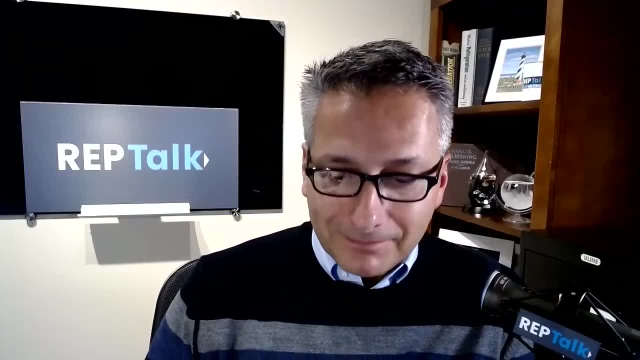 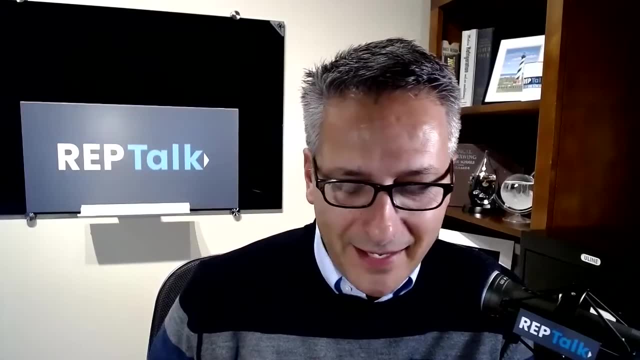 lot of money. you know bottled water is not cheap, right. And paying for healthier lifestyles- right. You know it's usually the good stuff that's not inexpensive. So if we try to eat healthier- you know healthy foods tend to be more expensive- We try to get a gym membership. 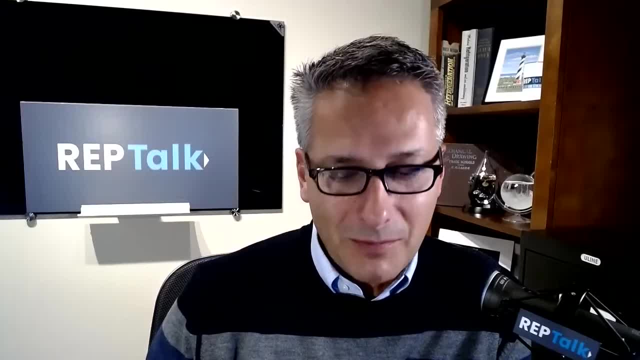 They're not always the cheapest things in the world. We try to live healthier, and it actually costs more money, right? So why not put a little bit of focus and energy on the activities that we're doing? So what I'm going to do is I'm going to go ahead and I'm going to 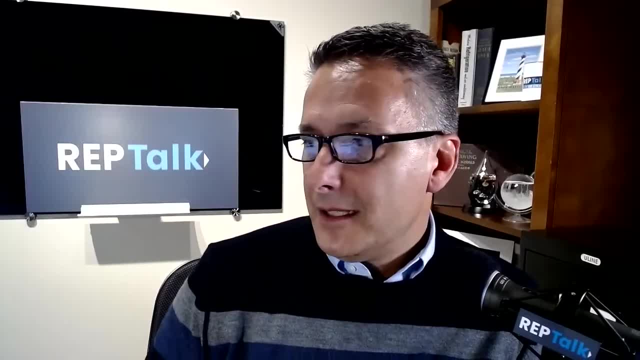 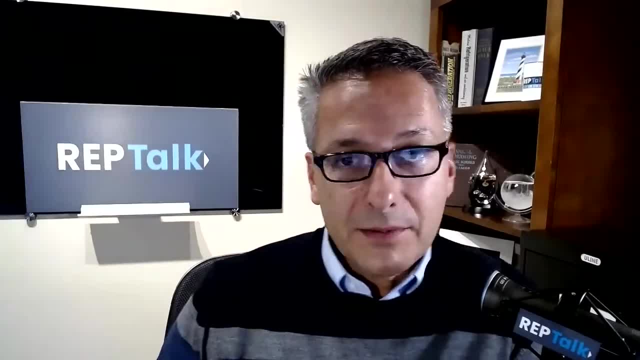 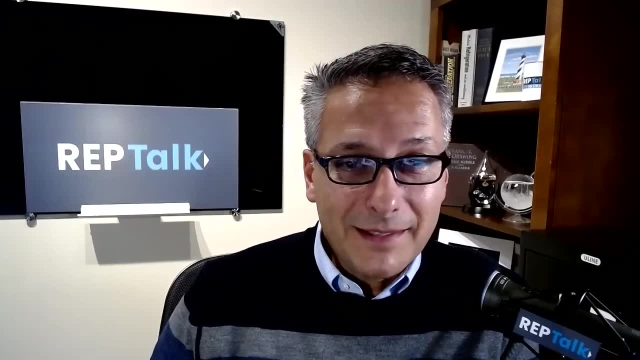 take in a day. I've not planned on giving up any single one of those. You know you have control over the number of meals that you eat per day. You need three, right? Or maybe you can give up one? eight glasses of water per day, Maybe I can give up one, but I'm not going to give up a single. 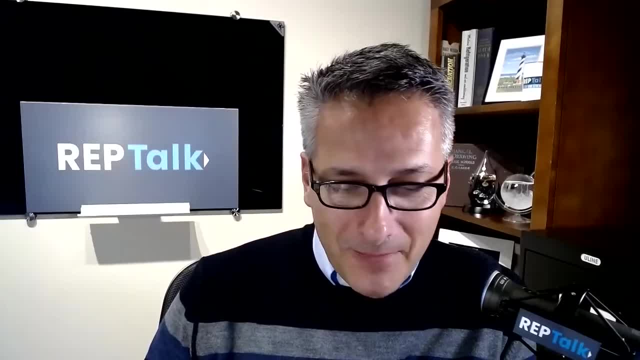 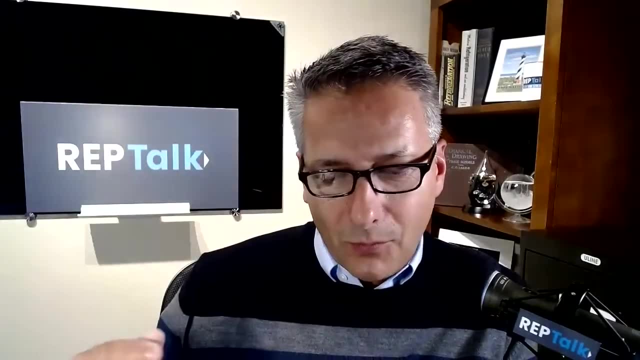 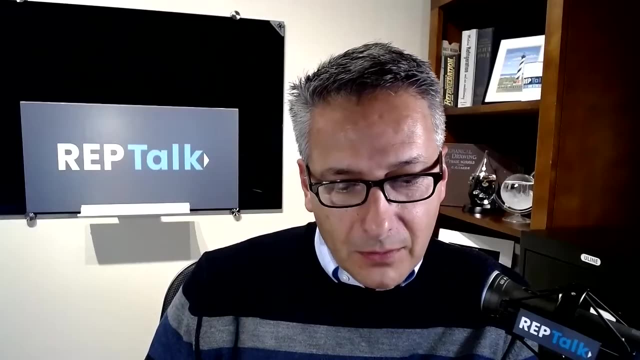 breath right, And I'm not going to not going to be part of the problem, although I'm not going to be part of the problem, although I am, just by sitting here, living and breathing right, We all are. So, anyway, what are we after when we want to clean or treat our air? Well, first of all, 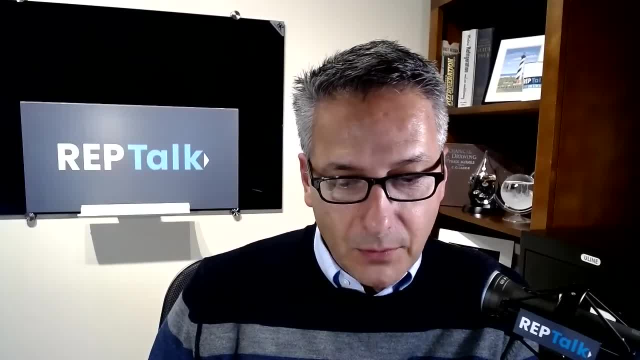 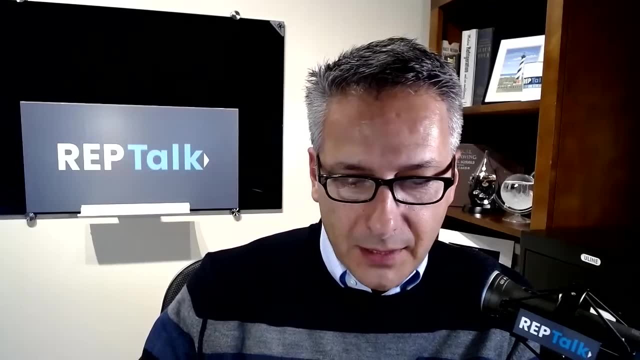 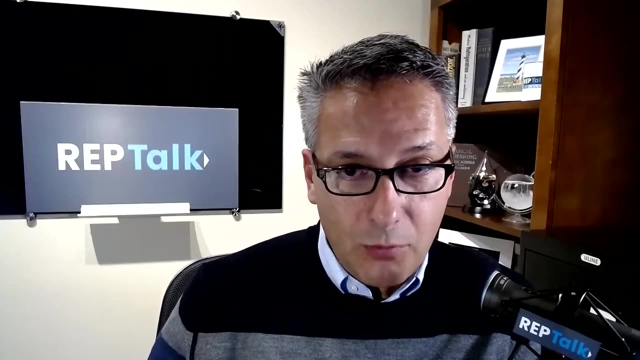 let's talk about whole home solutions versus room only solutions. If you could spend the money and you're willing to spend the money to get control over your air, it's worth. it's money better spent to take it at the whole home approach. 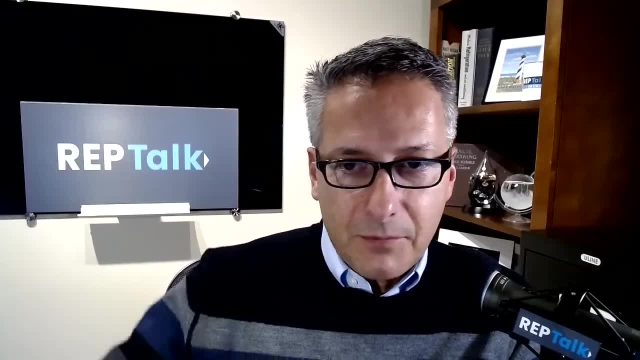 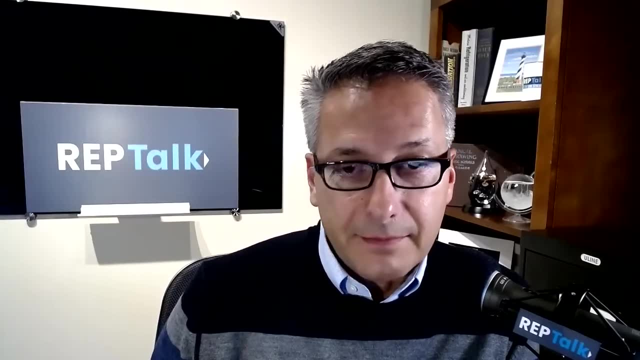 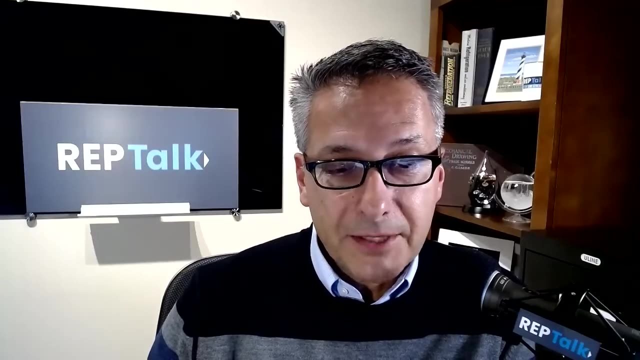 Room only solutions, like some of you might've seen some HEPA air filtration units that are room only. you know if they're worth their weight in gold they're. they're expensive And if you had to buy numerous HEPA filters it's going to add up very quickly. So I think it's money better spent. 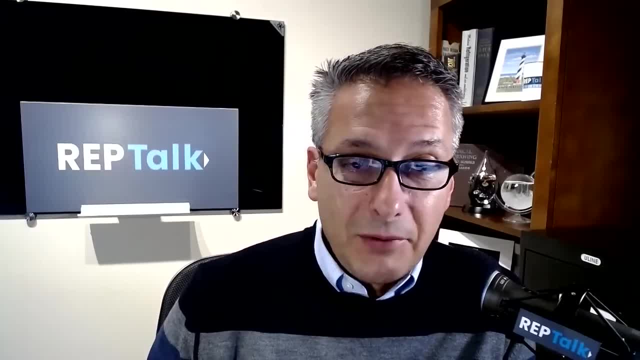 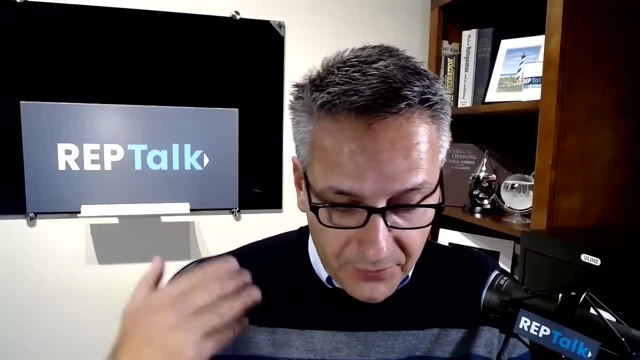 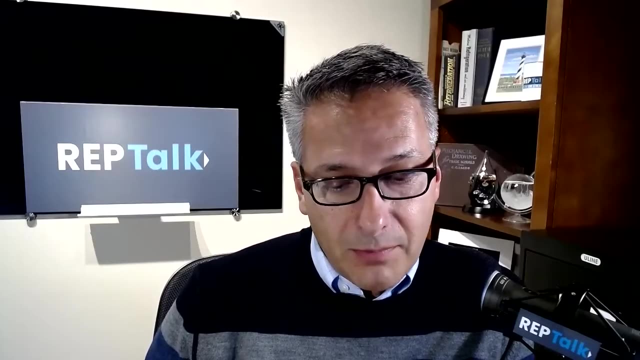 if you look at whole home solutions, that is, if you have a forced air system- In other words, there's a fan blowing hot air or cold air, depending on the season. There's, there's a fan in the system And you know it's forced air system- It's easier to do a whole home, take a whole home approach. if 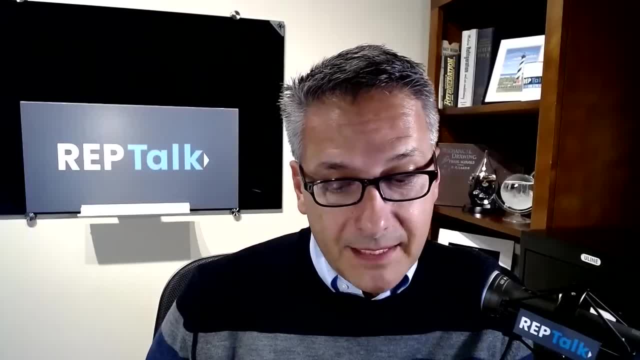 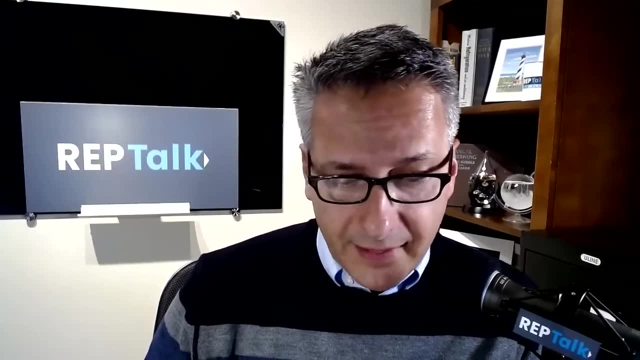 you have a forced air system. If you don't, you might have a hydronic system, steam or hot water boilers, which is great, you know, great for heat And you know obviously you're not blowing things around like you do with a forced air system, But there you might have to take a limited room only. 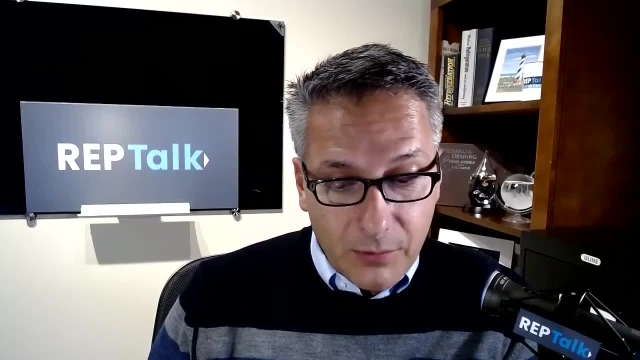 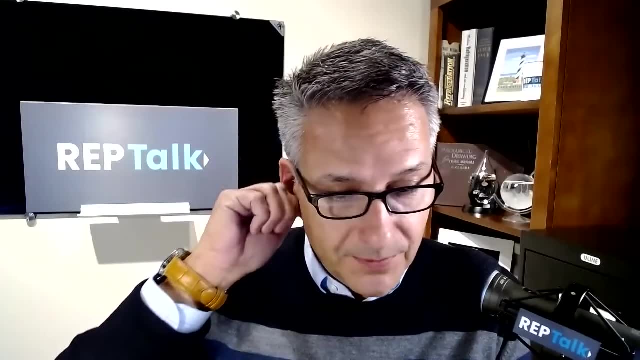 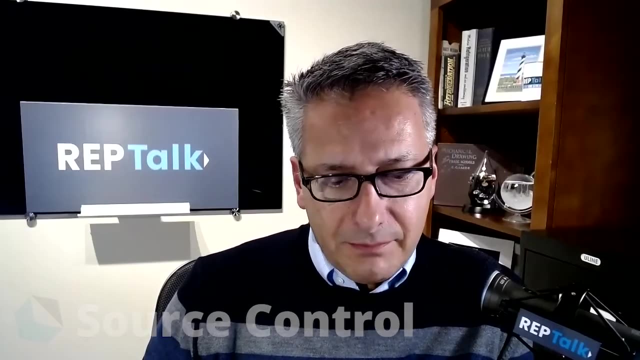 approach, But it is always possible to add duct work if you really wanted to, to have some, you know, some wind and water and all these other strategies we're talking about. So, anyway, think in terms of whole home solutions. First, I'd like to talk a little bit about source control. Alright, 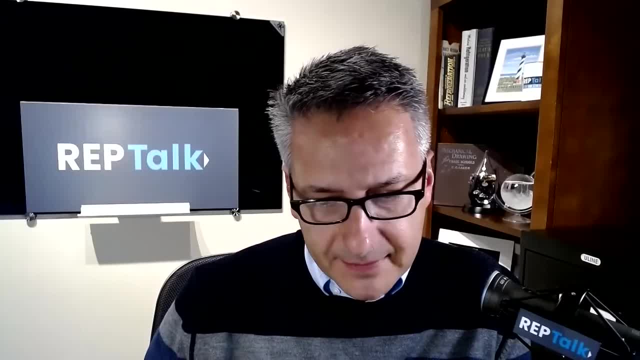 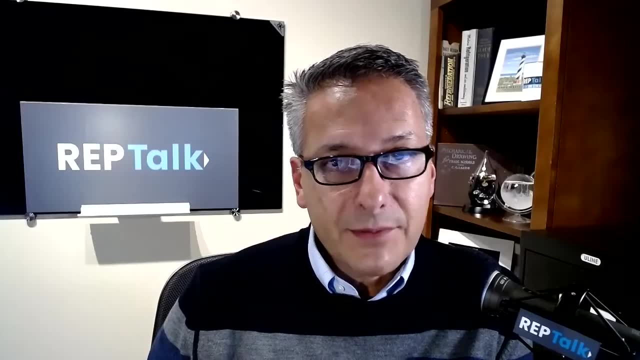 this is kind of taken on a new meaning during the past few months, during this pandemic, because you know, I'm sure everyone has heard by now about, you know, hand and surface disinfection right, Washing your hands for 20 seconds, washing surface spaces right. So when you go to a restaurant or a. 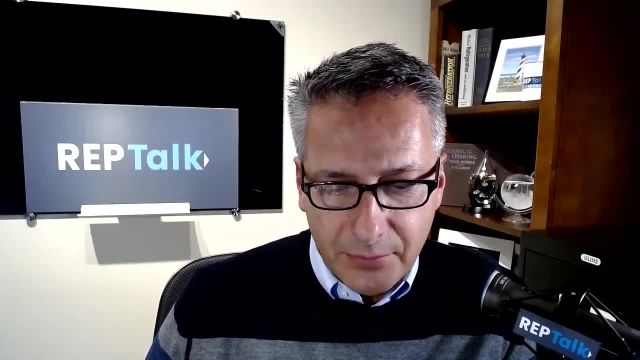 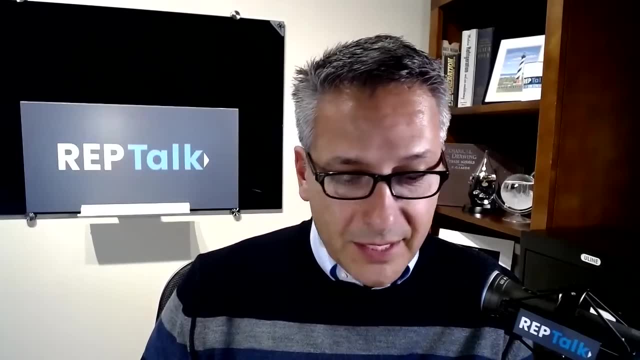 hotel. now you know, for these cleaning procedures and protocols is to make sure the germs are gone and we're keeping you know our touching surfaces are clean. Traditionally speaking, you know the same rules apply for your house- good housekeeping right. You want to keep those cleaners and 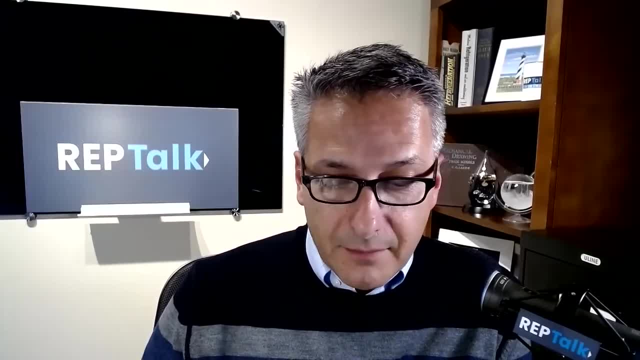 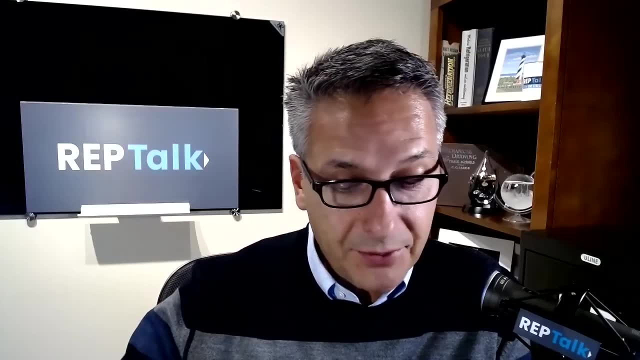 chemicals isolated. That is an approach. There's some folks out there with hypersensitivity to those chemicals and you would actually have to store those outside. Maybe you have a detached garage and you would actually put them outside, So isolate those chemicals. Maybe you don't have. 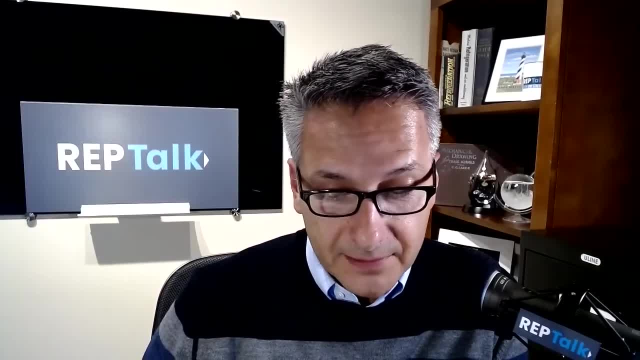 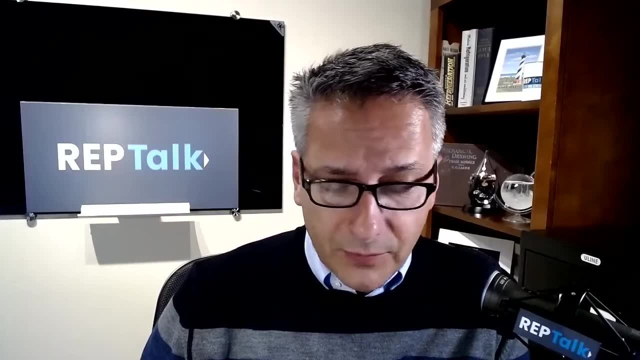 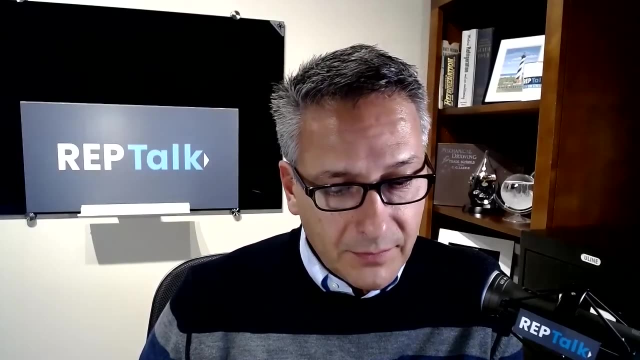 a detached garage, but keep them out of your breathing space, out of your house, if at all possible. You want to fix any water leaks or issues. wet basements come to mind, roof leaks. take care of those, because water will become and is a perpetual source of creating certain issues. 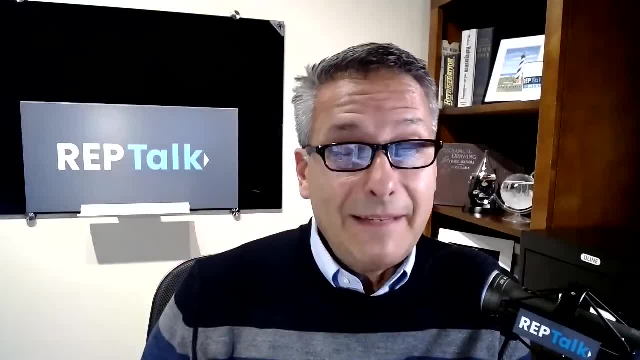 like mold growth right, So take care of those. You want to keep insects and rodents outside the house. You want to keep insects and rodents outside the house. You want to keep insects and rodents outside the house? Keep them out of your living space. Make sure you get everything sealed. 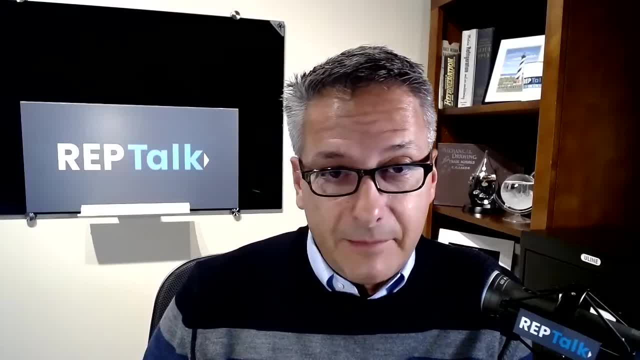 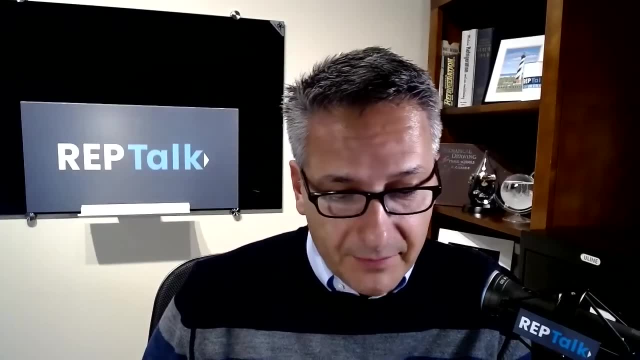 up. Problem with them is what they again. what they leave behind, just like the dust mites, is very allergenic and is a problem for people with allergies. We definitely don't want to be breathing in whatever they're leaving behind. I would like to add to that a little bit by making 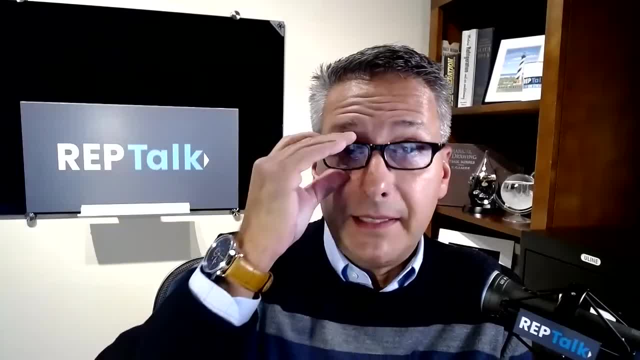 sure that your kitchen and exhaust fans are working properly And if you have a kitchen hood over your stovetop or cooking surface, make sure that you have a kitchen hood over your kitchen hood over your stovetop or cooking surface. Make sure that you have a kitchen hood over your. 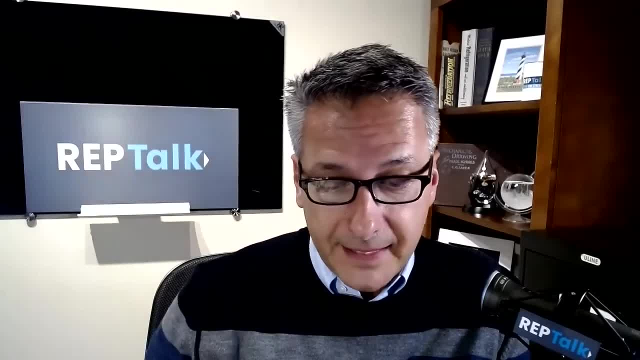 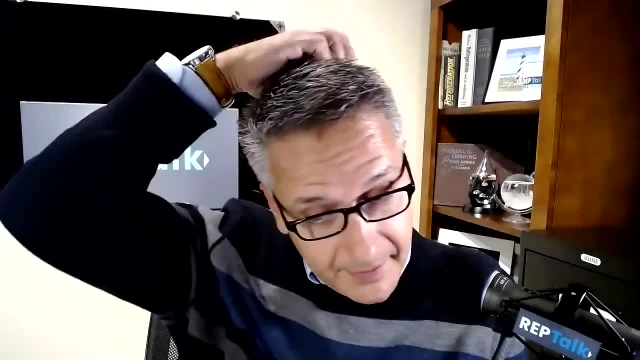 venting outside if at all possible and not recirculating in the space, because a lot of VOCs are given off just during the process of cooking. So think about that. Maybe you can have it ducted outside And make sure the bath exhaust fans are working properly, because humidity 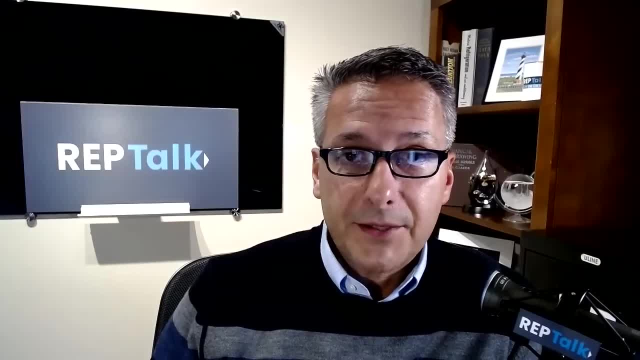 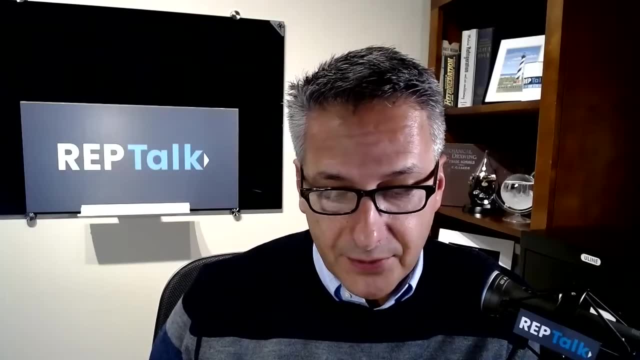 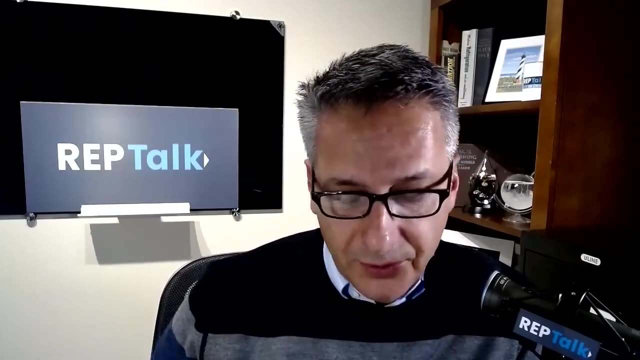 excess humidity and moisture do, like I said before, they create issues. They create mold growth and cause situations where it's really not good for, and you can have a reaction to mold when it grows. obviously Most people actually can. So source control is number one. Second one I'd love to talk about is air dilution. Air dilution- 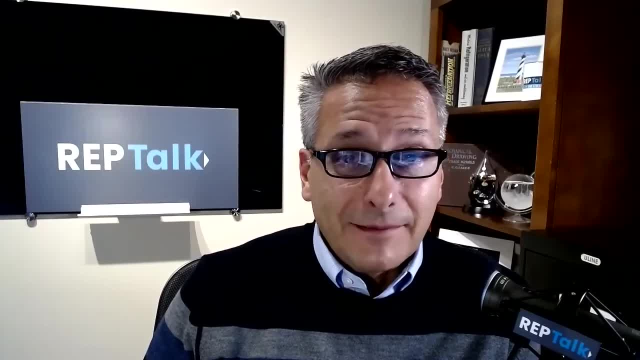 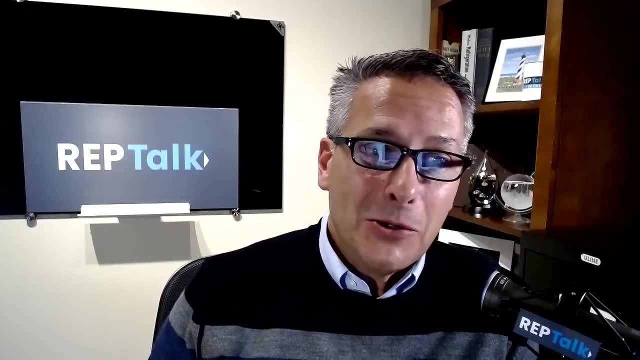 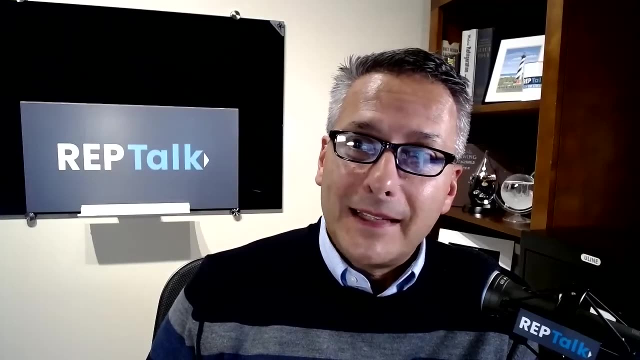 is fresh air. Fresh air is often, very often, underrated. You know, it'd be great if we could keep the windows and doors open in our homes throughout the entire year, but most places you can't right. So when you close up those windows and doors the air in our spaces tends to get more. 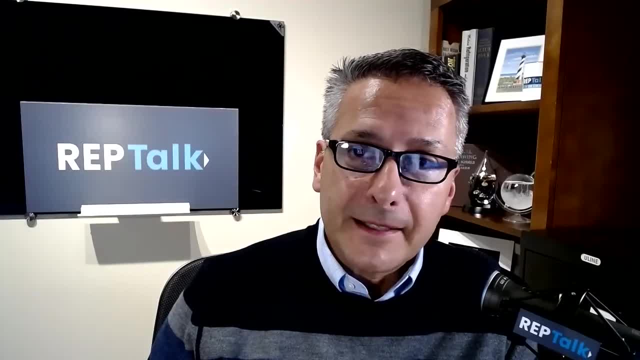 polluted? if it's not, you know, if you're not letting fresh air in. So if you're not letting fresh air in, you're not letting fresh air in. So if you're not letting fresh air in, you're not letting fresh air in. So if you're not letting fresh air in, you're not letting fresh air in. 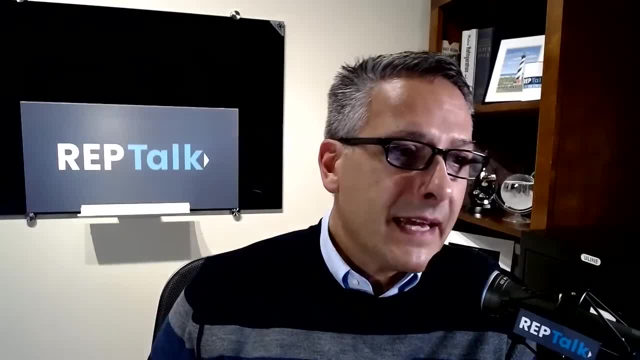 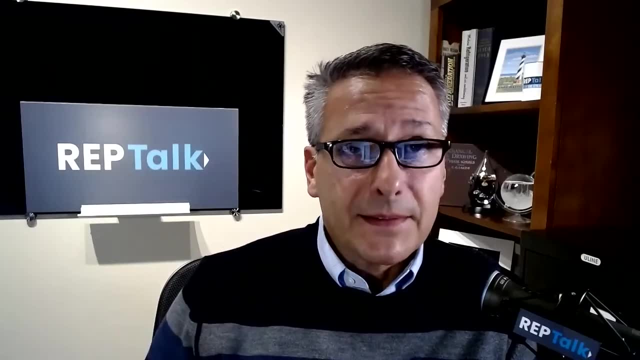 And the EPA has done studies on this and found that the average indoor breathing air can be two to five times higher, higher, more polluted, than the air outside, in some severe cases, over a hundred times more. So, again, fresh air is key. So when you can't open those windows and doors, what do? 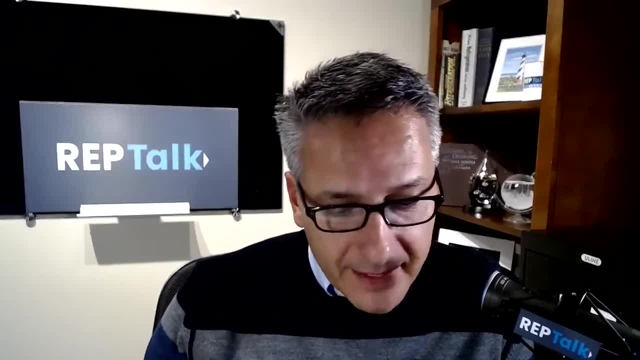 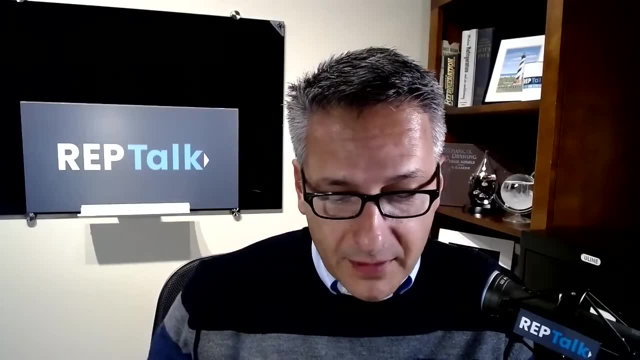 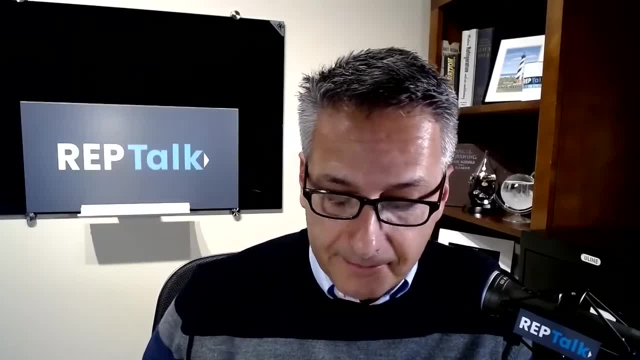 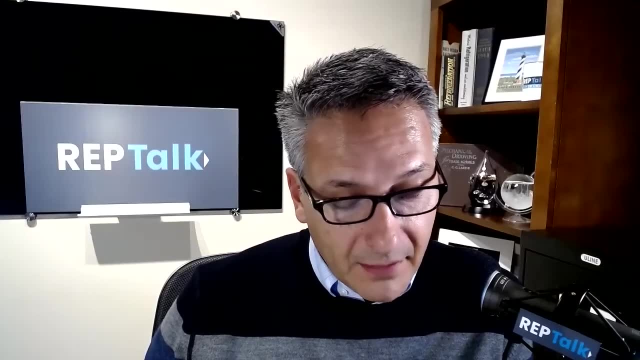 website. go to the website, go to life breathcom and click on the homeowners tab And there's a great little video and description on there about what the difference between a heat recovery ventilator and an energy recovery recovery ventilator is. basically, we're talking about a. 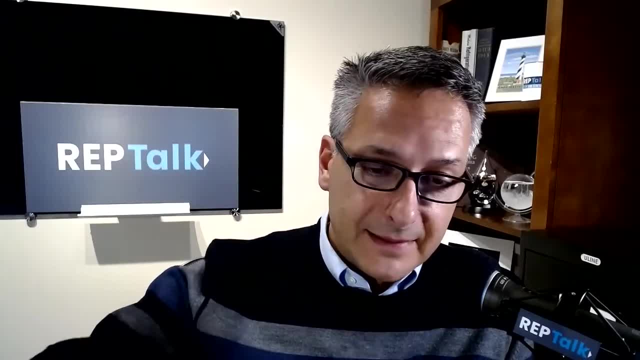 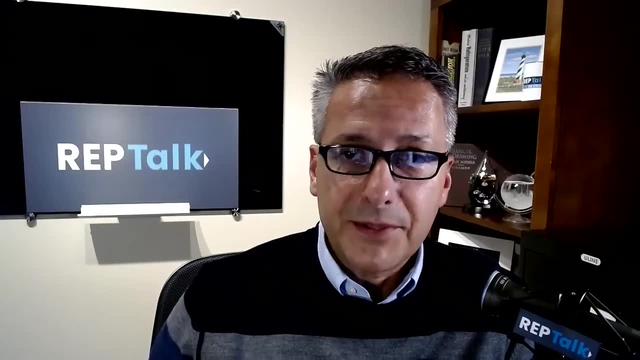 box with two fans in it. You bring- uh, you exhaust the stale air out of the space and simultaneously bring in a fresh air replacement for that stale air. bringing fresh air, and you temper it before it goes into your main heating and cooling system And you typically leave those. 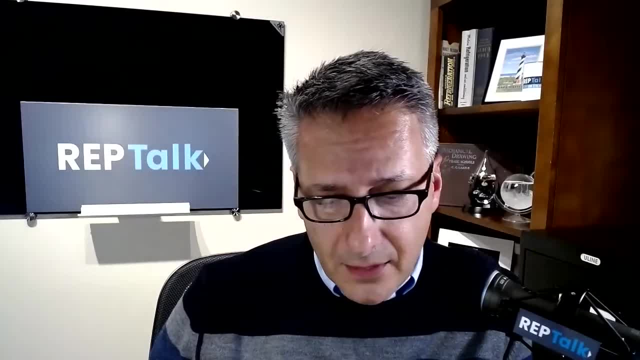 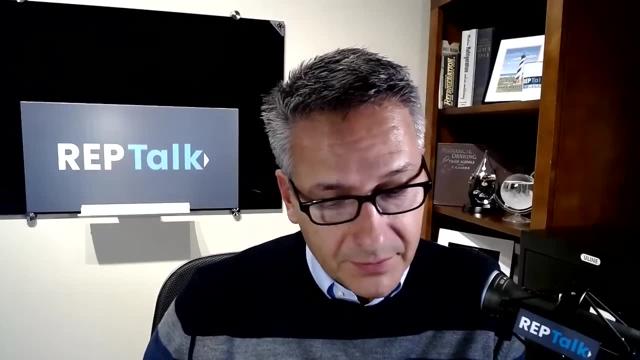 on all the time and occupied or when you're home, Um, and they're very energy. most of them are very energy efficient. So you're constantly getting that fresh air And in those months where you can't have your windows and doors open. So, again, bringing fresh air in is key. I myself, I live in- 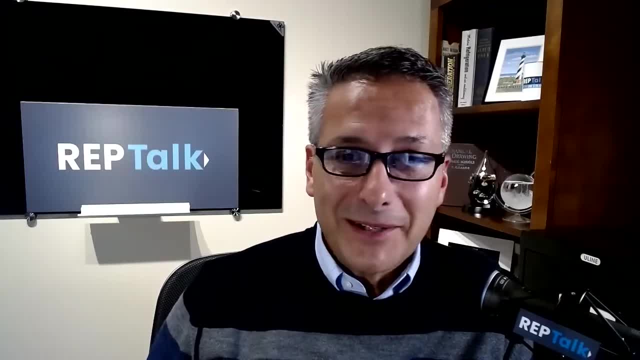 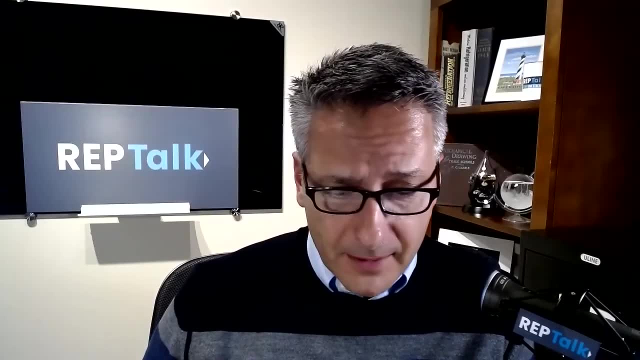 a Northern climate, I typically will open my windows in the dead of winter just to bring some fresh air and air the house out. I do air the house out. If someone is sick in your house and has a cold flu or um something worse, God forbid, um, you know, think about having them in a room. 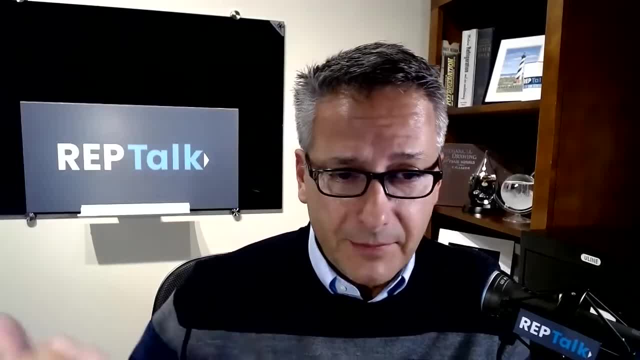 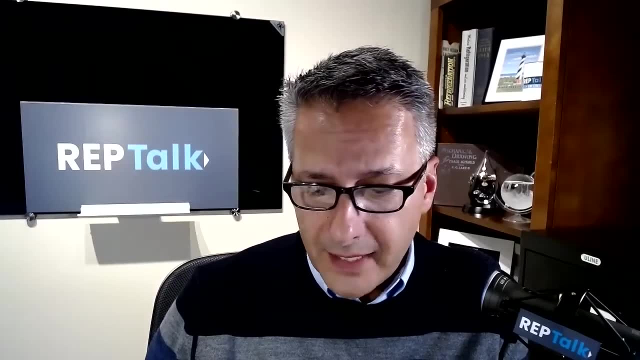 and cracking the window in the room and maybe having the bath exhaust fan on just to keep the fresh air and circulating and keep others from potentially getting sick as well. It'll limit that. studies have shown fresh air does goes a long way to um helping those folks get better, um and 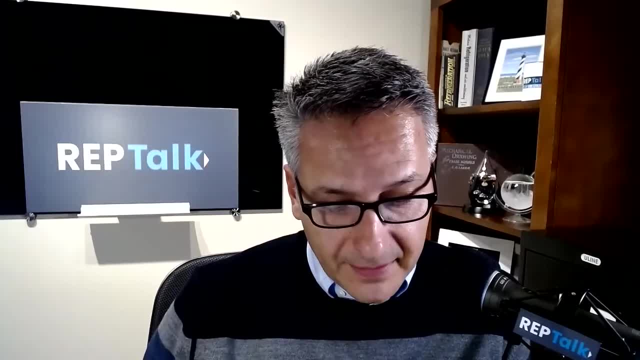 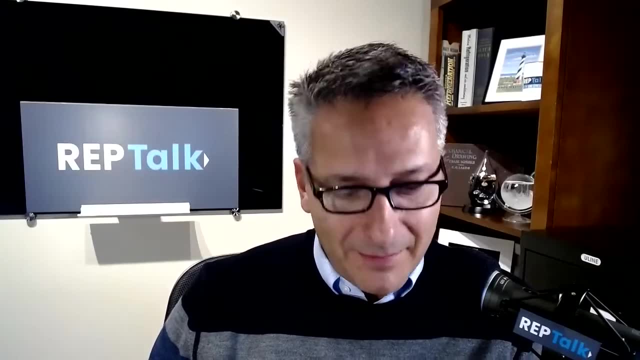 keeping anybody else, uh, the chances for anybody else to get infected as well. So air dilution, uh, dilution is the solution To pollution. Remember that. How about there's a? there's a good golden nugget for you. 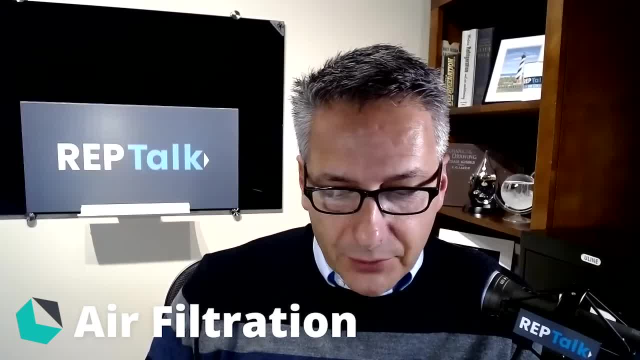 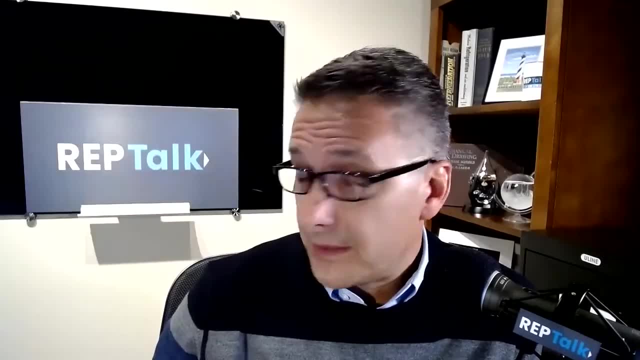 Next, I'd like to talk about air filtration. right So, air filtration. you know what an air filter probably looks like. Most of them are one inch. I think half the market is a one inch air filter in our homes, uh, throughout the homes in the U S. a lot of them are throw away or disposable. 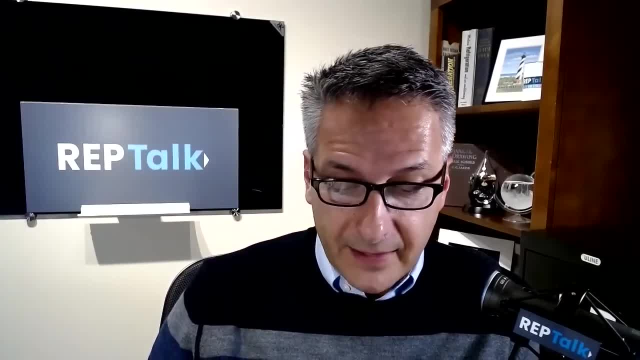 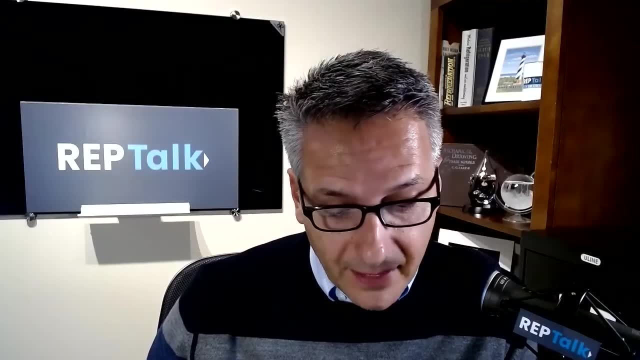 type air filters. Um, they're meant to help remove particulate out of the air. If you're using a one inch air filter or disposable type air filter, there's probably room for improvement in this in this area. Uh, most hardware stores that you might get your filters at they're not those, those filters that. 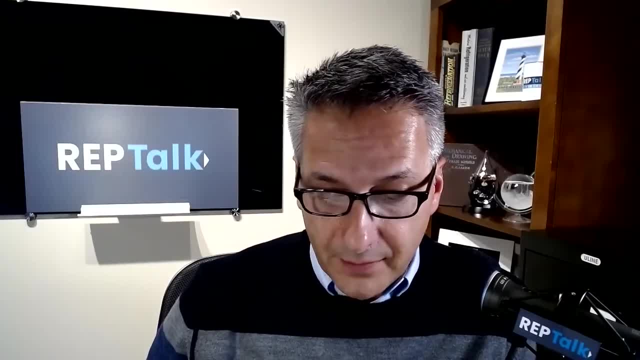 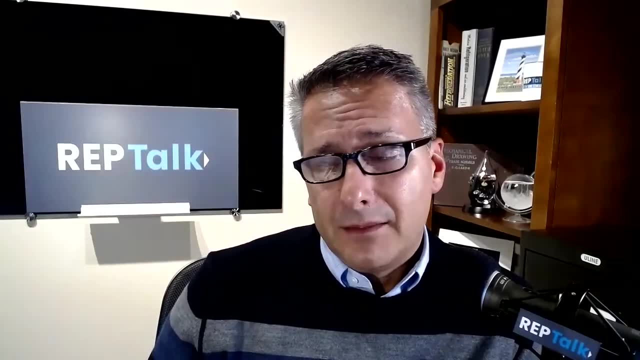 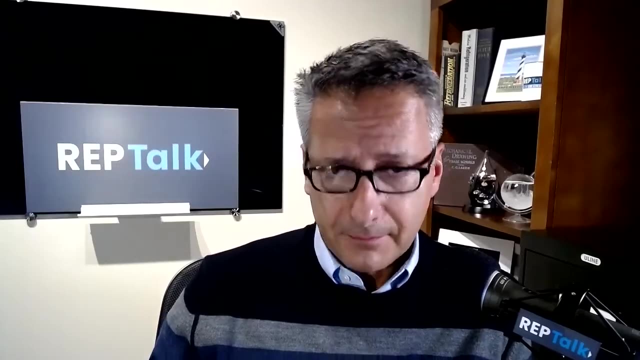 they're selling typically are not capable of improving the filtration in the house. You want to get something that's got a deep pleat, three or four inches deeper pleat, And that usually they come with their own cabinets. Um, if it's um, you know, a forced air system where that one inch 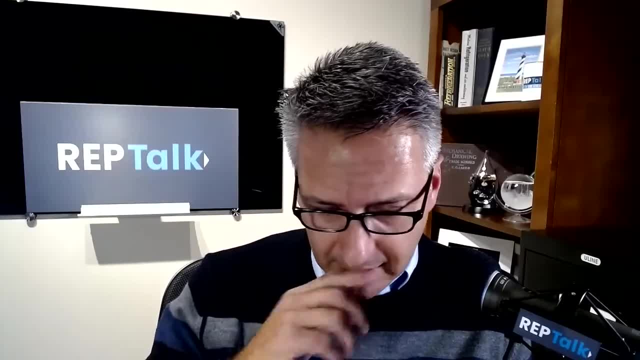 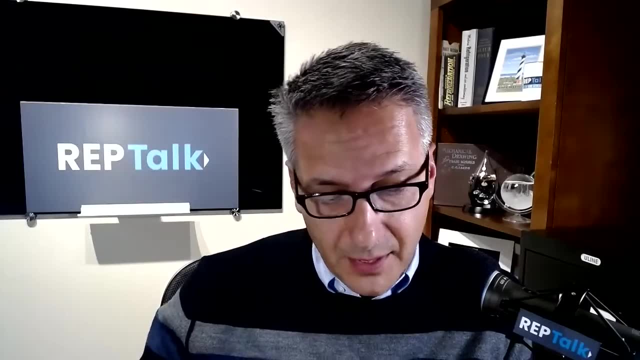 slot is right now. the duct work would have to be modified to include, uh this media air cabinet, Uh with a higher, uh, higher Merv rating. we call it a Merv rating, which is a way to measure the. 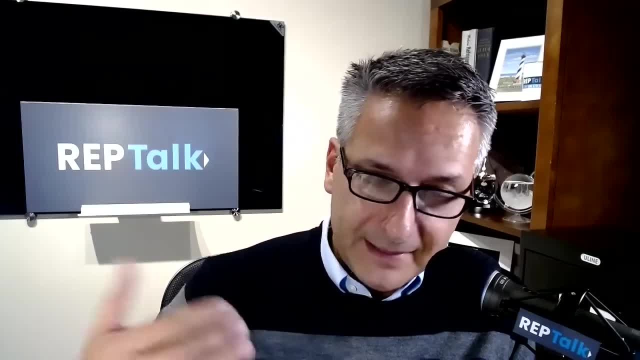 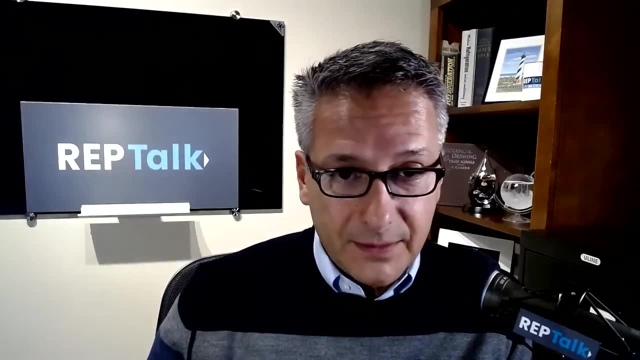 amount of particulate a filter can remove out of the air. It's basically a scale of one to 16.. The higher the number, the more it takes out of the air. Most of those hardware stores that sell those go up to about a Merv eight, about halfway down the scale, but 11 or higher is what you're. 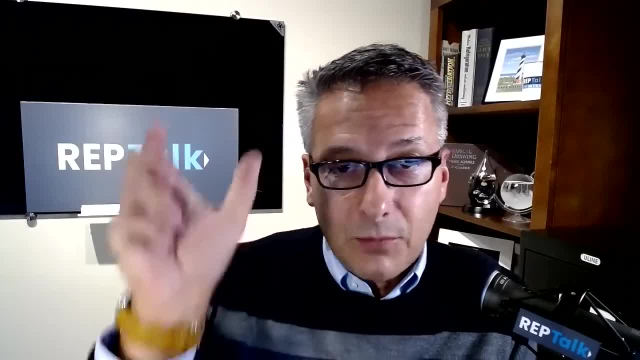 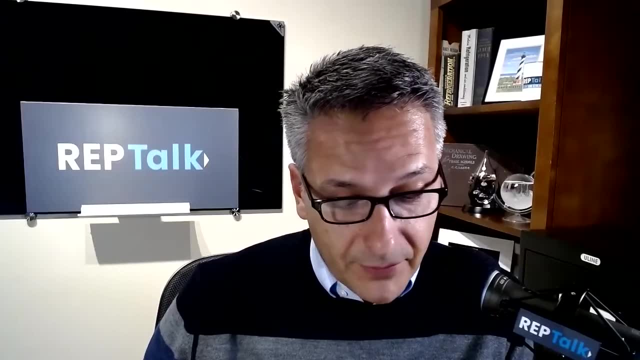 targeting. If you have return air filter grills, where there is a one inch slot in a grill, uh, there's solutions for that as well. Uh, and we can. some of those could be a Merv 11 or a Merv 13 too, Both ASHRAE, uh, which is the. 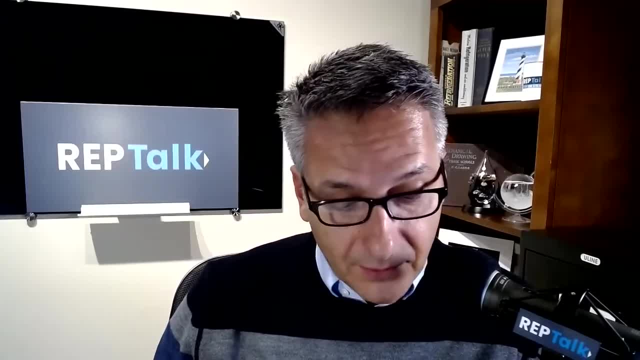 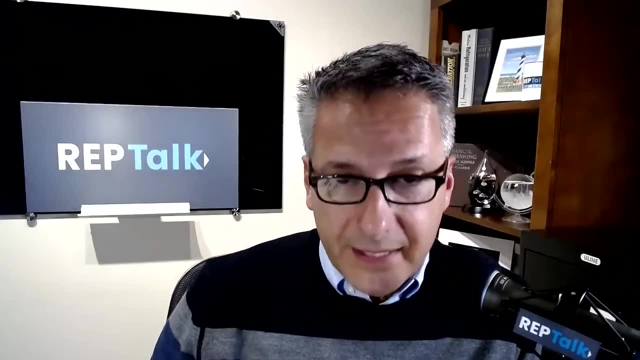 American Society of Heating, Refrigeration and Air Conditioning Engineers, along with the EPA, recommend Merv 13.. So you might've read or heard about that over the past few months as well. Merv 13 does a great job of addressing some of those droplet. we call them droplet nuclei. 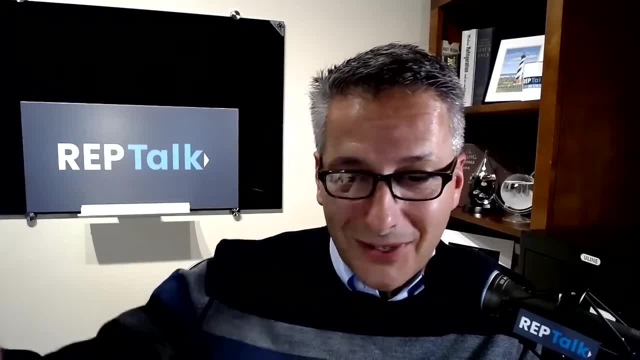 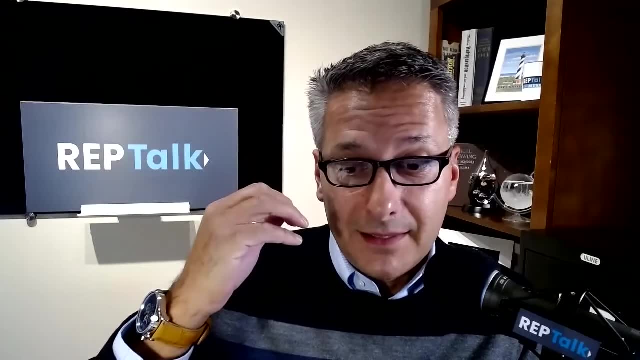 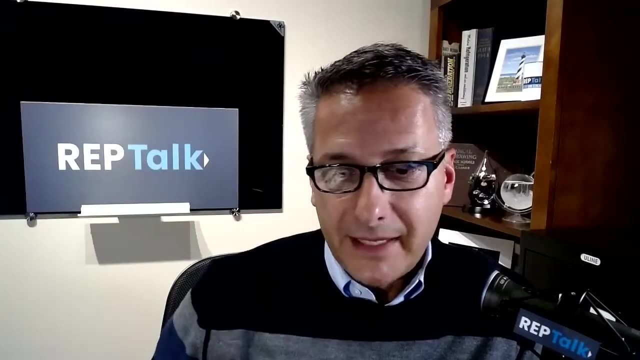 the suspended uh infectious aerosols. Sometimes they can be infectious if if there's um, um pathogens, They can be infectious if they're not associated with them. And then we're talking about sneezes and coughs. So when somebody sneezes or coughs it, you know, inject this droplet nuclei into the air. 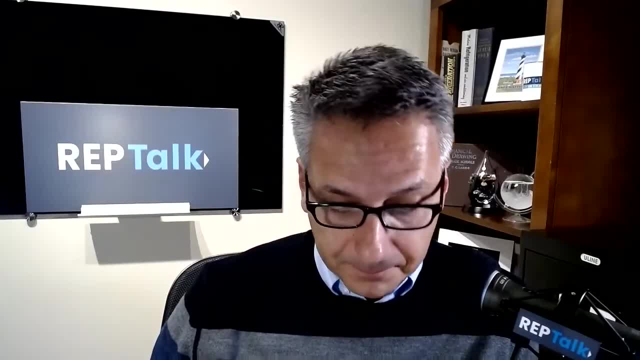 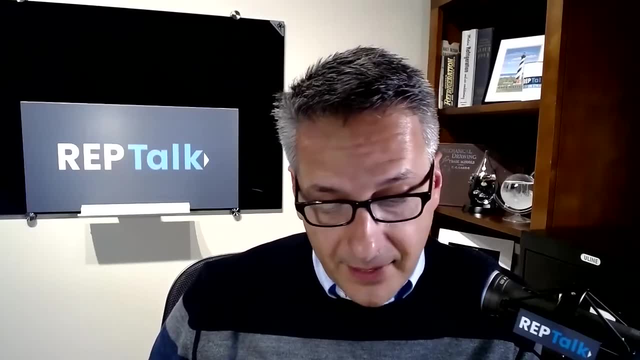 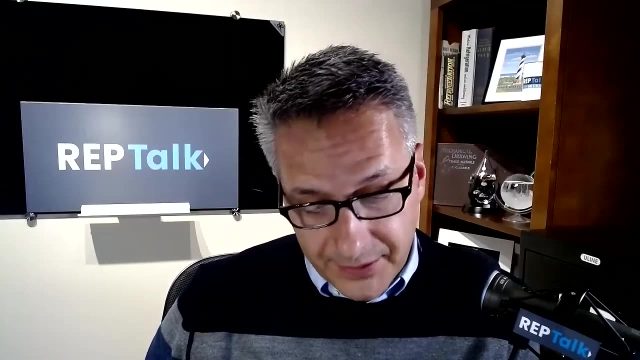 and Merv 13 goes a long way to getting and reducing that droplet nuclei in the air. Um, there are uh solutions to even go above Merv 16.. There's what we call HEPA air filtration. HEPA is high efficiency particulate arrestor, or what I call hospital grade air filtration. 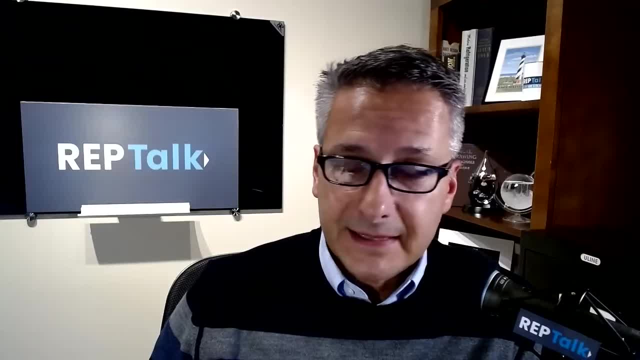 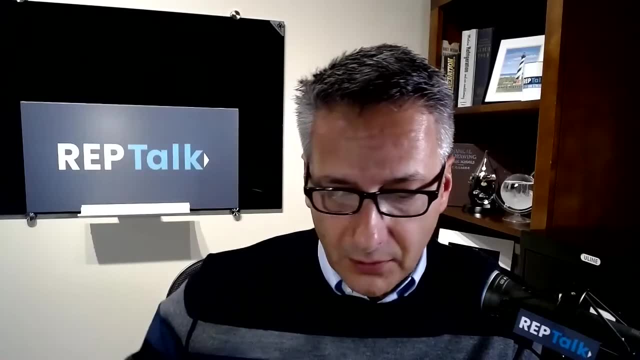 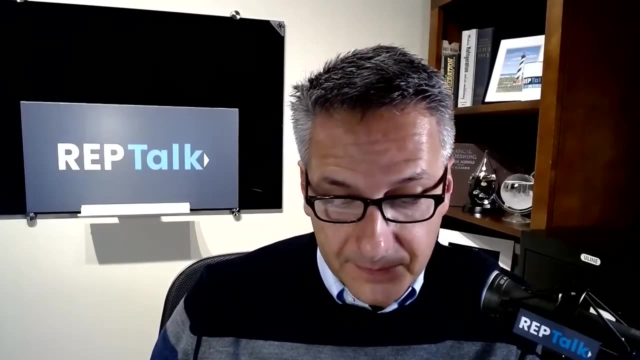 Um, HEPA filters are available in your home. There's a whole home HEPA air filters available that can attach right under your existing ductwork. uh, in a matter of a couple of hours, there's a fan in there um to help assist the air filter to work along in conjunction with your main fan in your system, um, and you can actually have hospital grade air filtration for your house. 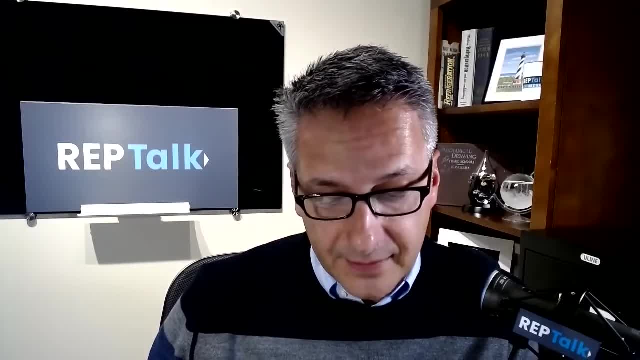 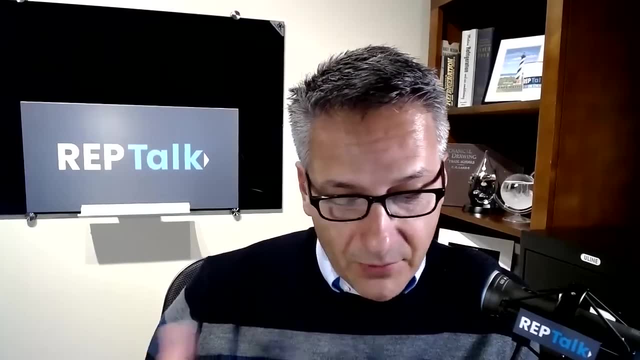 So keep that in mind as well. Uh, HEPA filtration is is available for the entire home, not just the room mounted Um so that. so for air filtration again, the higher the Merv rating. look into deep pleat. 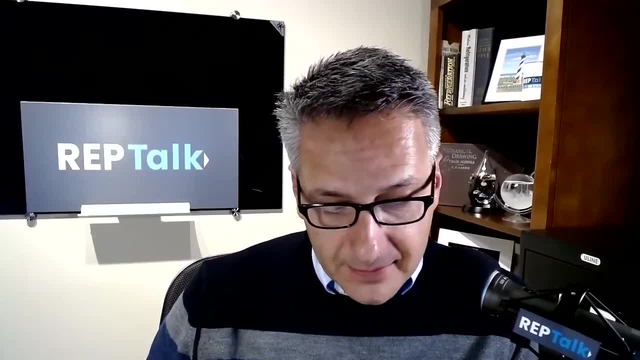 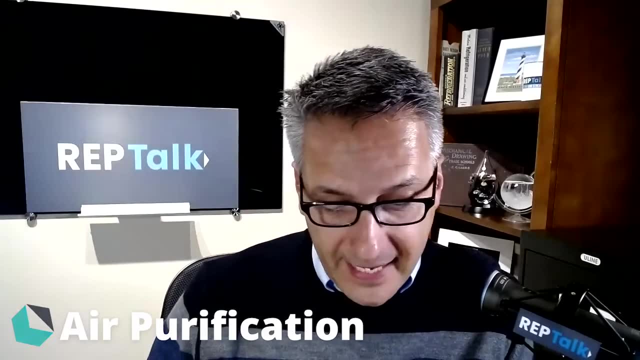 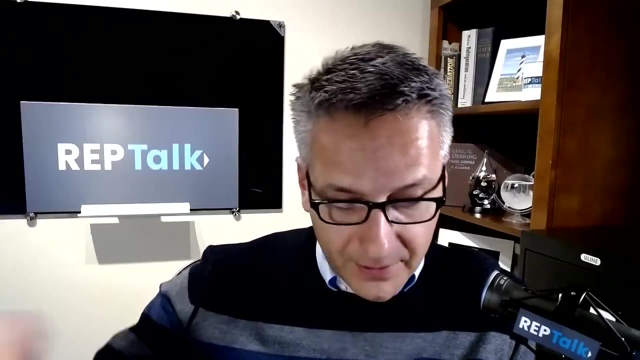 air filters. uh, that'll go a long way to uh taking a step in the right direction. Um, I'd also like to talk about air purification. So what can you actually do, mechanically speaking? install a device to help actually treat your house and the germs and the odors and particulates in it. 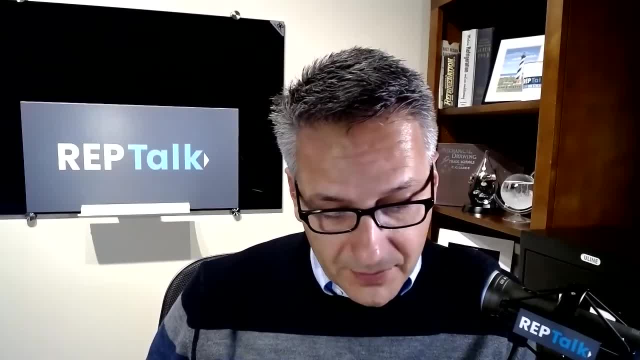 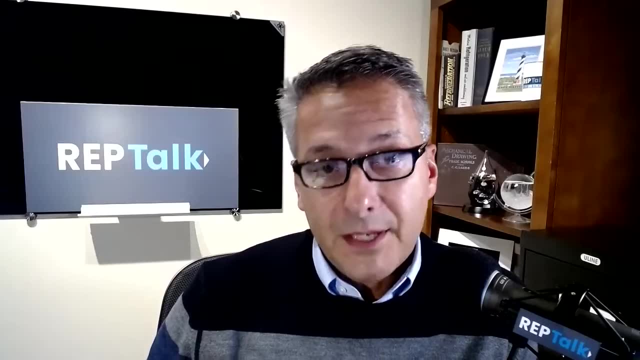 So there are devices on the market that are whole home devices that will treat all three levels of contaminants that we mentioned- the germs, odors and particulates- and treat the entire space Using your air distribution system, So your ductwork and your registers and grills. 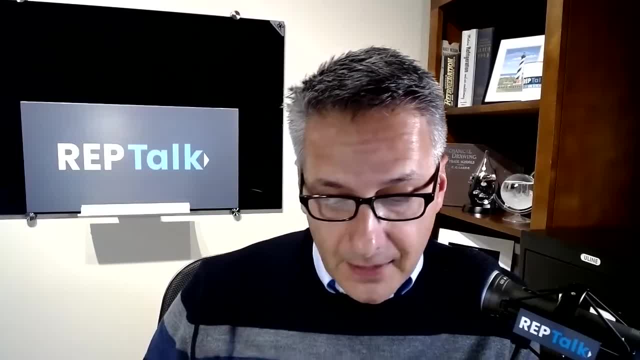 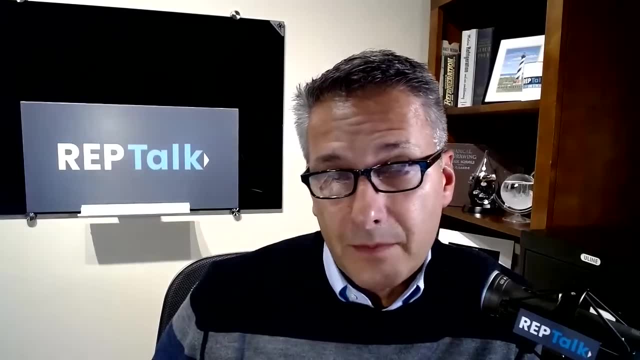 um to uh, to treat the entire space Um. what I would say is key here is: make sure you find a device that's third party tested and has its technology proven by a third party so it's been validated, so they can back up what they're saying that the device actually does. 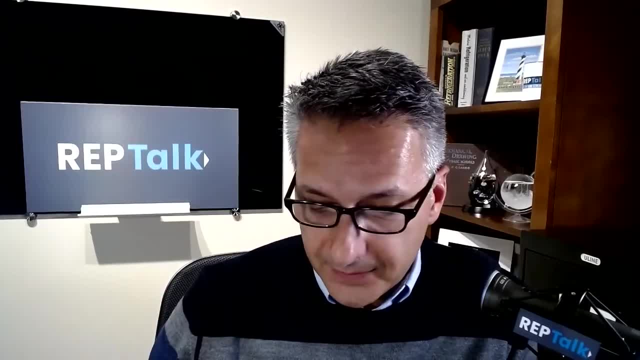 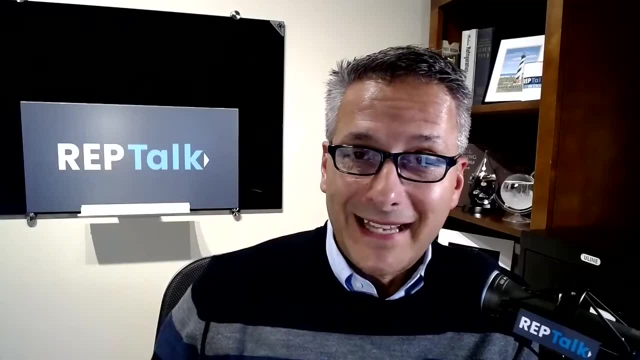 Um, so please find a device. they're out there. There are solutions out there that are third party validated and can treat the entire space proactively. And look for one that not only treats the air that we're breathing but also surfaces. So if I, if I'm sick and I touch a, 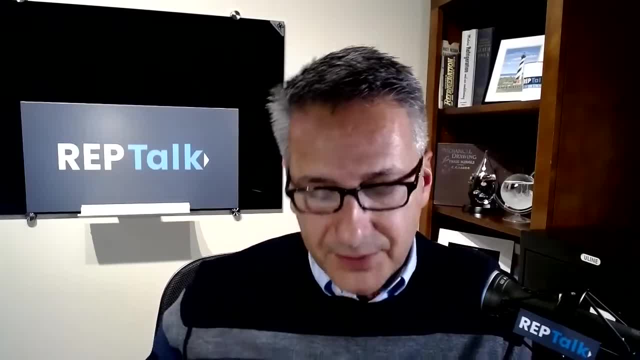 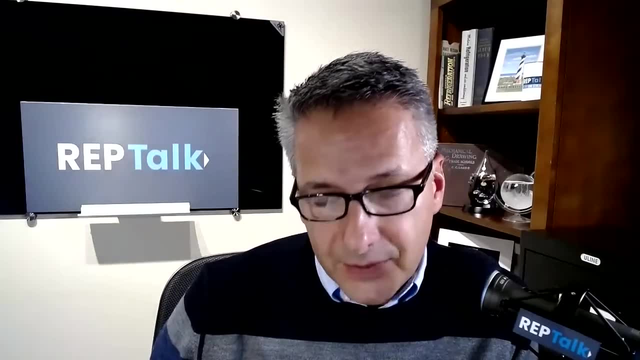 surface. somebody could come along behind me and my family or whatever touch the same remote control that I would just touch, Um, and there's a potential for them getting sick too. So find a device that actually will treat all three levels of contaminants and not just treat the air. but 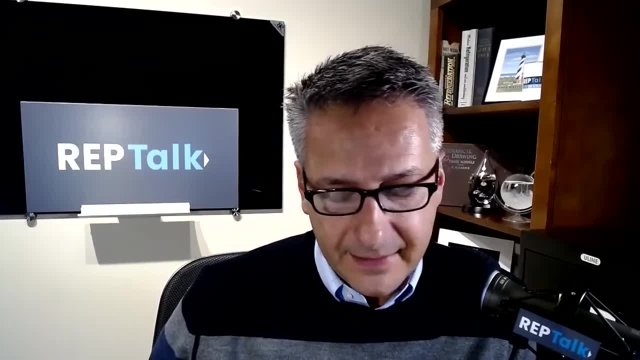 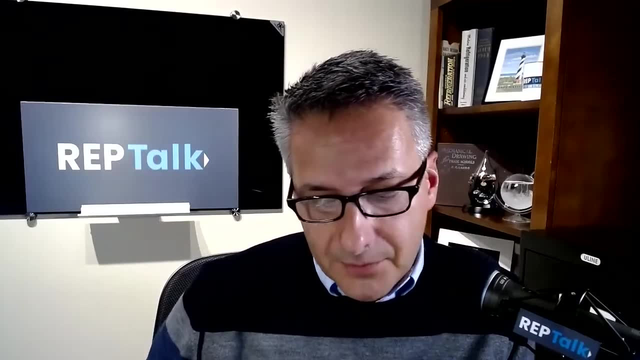 the surfaces as well, And I would think of all the things we touch. you know, like I said, remote controls, keyboards, telephones, kitchen counters, uh, the refrigerator door handle? Um, so, find there are, there are solutions out there for whole home air purification. Lastly but not least is 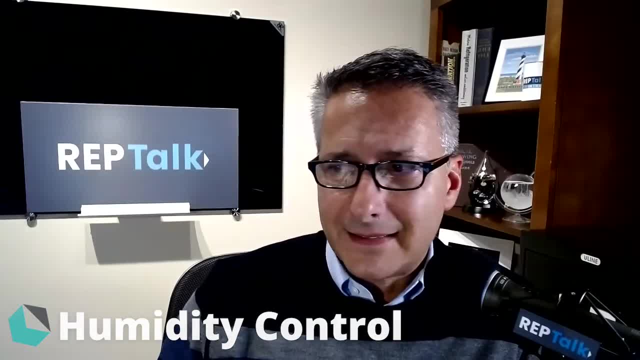 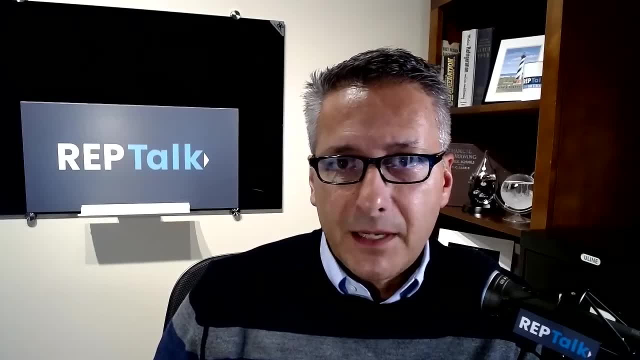 humidity control. This, this, this conversation has gained more depth over the past few months. you know, and usually in in the heating and air conditioning trade, we talk about humidity for comfort. It's changing. The narrative is now changing because of the studies that have been. 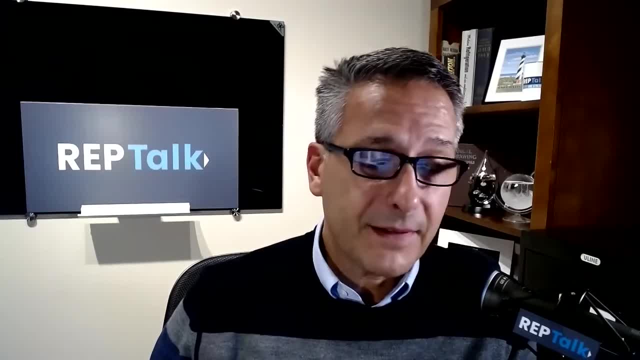 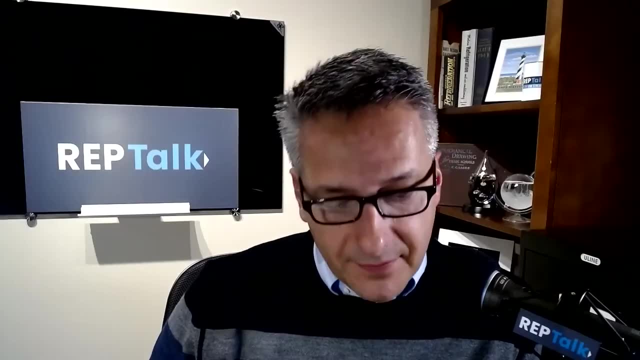 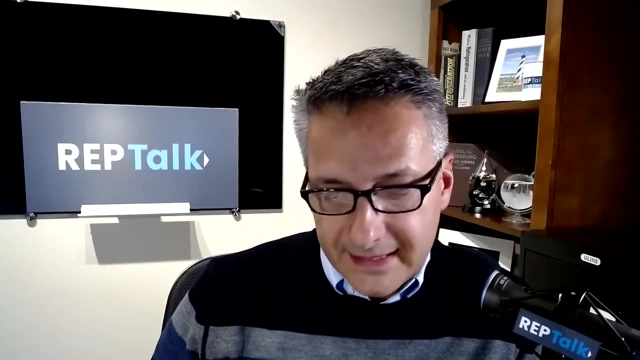 done Shown on humidity and its effect on the pathogens and effect on our bodies and how we react to those pathogens. Um, and if what we found is, and those studies found, is if you're outside of the optimal healthy range, which is 40 to 60% relative humidity, if you're outside of that range, 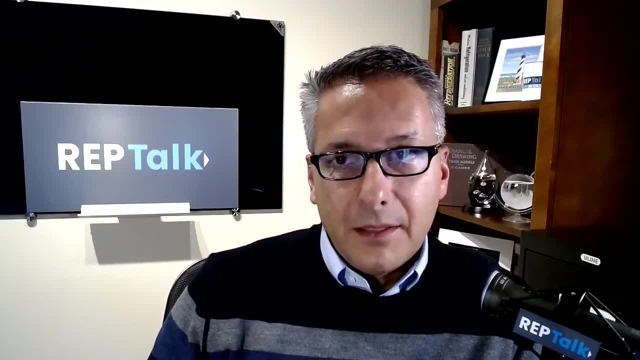 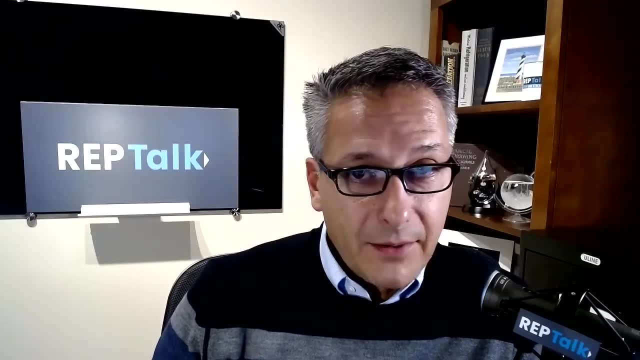 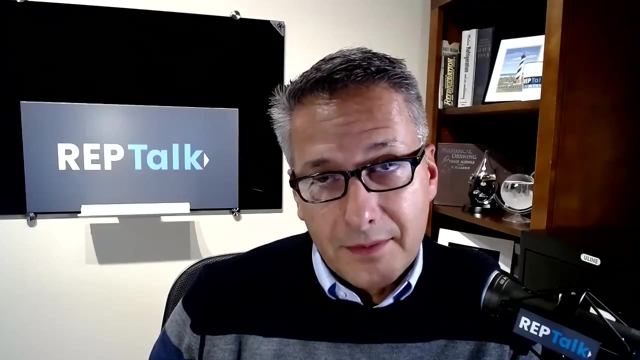 two things can happen. A, you're going to enable pathogens to survive longer. Okay, The dryness The air or the more humid the air, uh, they can last longer. And B- um, the other thing that can happen is, if you're outside of that range, you're going to actually limit your body's ability to 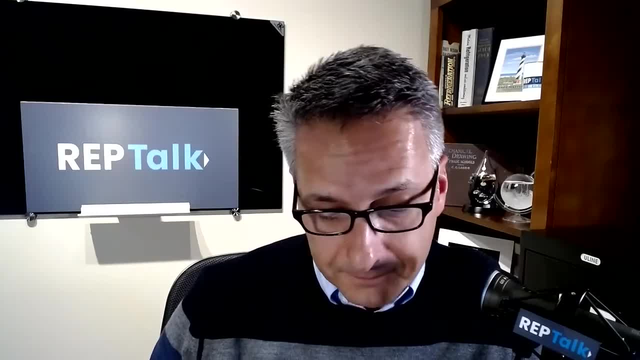 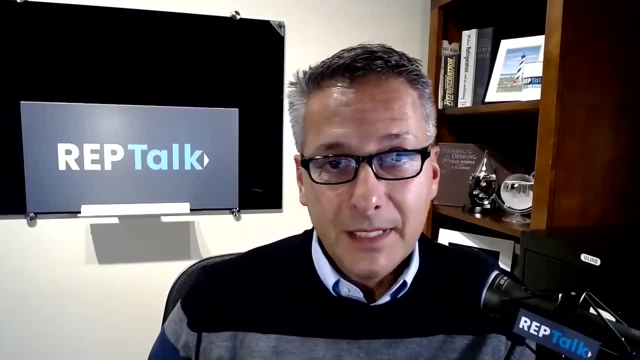 fight those pathogens. Okay, So keep that in mind as well. So remember: 40 to 60% relative humidity. Now what do you do about that? How do you control humidity? You know your heating and cooling system is primarily for sensible, uh, heat, which we call what you actually feel right. So you have. 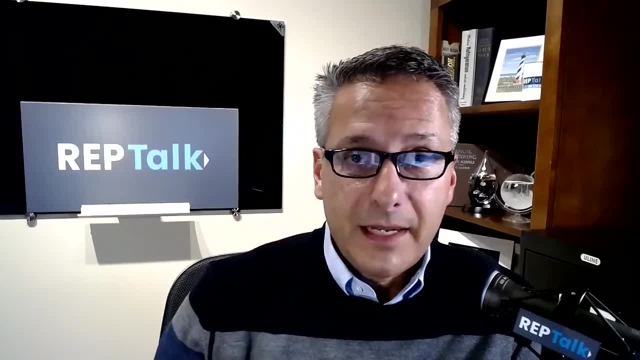 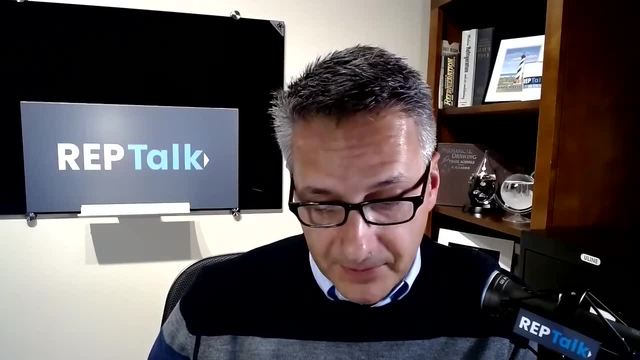 the thermostat. you turn the thermostat on. you turn the thermostat on. you turn the thermostat on up and down, depending on how you're feeling- hot or cold. right, Humidity does, uh does, have an effect on how you feel, comfortably speaking, but your system is not typically designed to address. 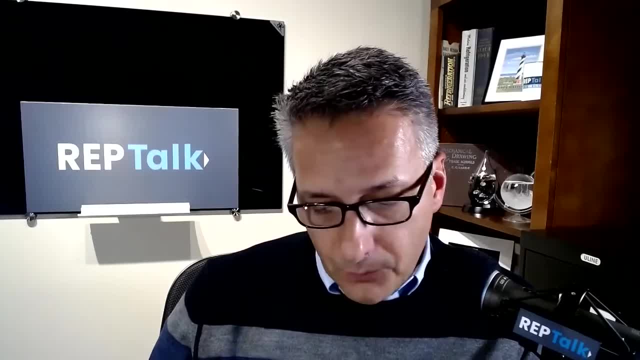 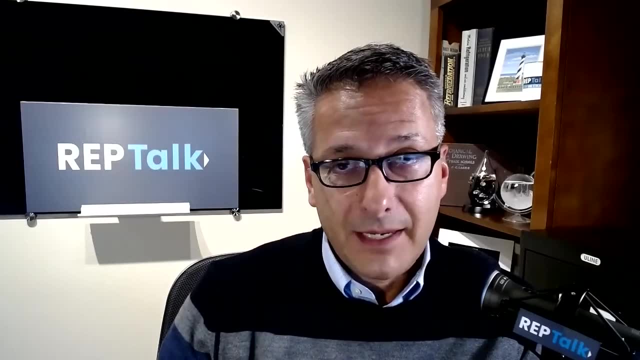 humidity directly. Okay, What do I mean by that? So if you live in a Northern climate, you run your heating system. We tend to dry the air out. Okay, With the heating system operating, we tend to dry the air out and you can easily, easily fall below that 40% relative humidity. So if you live in a Southern climate, you're not doing anything. I think we tend to run around 20, 20% relative humidity without doing a thing, So you need to bring that back up. So you would add on a whole home: uh, humidifier. Uh, there's different types of humidifiers There, actually.